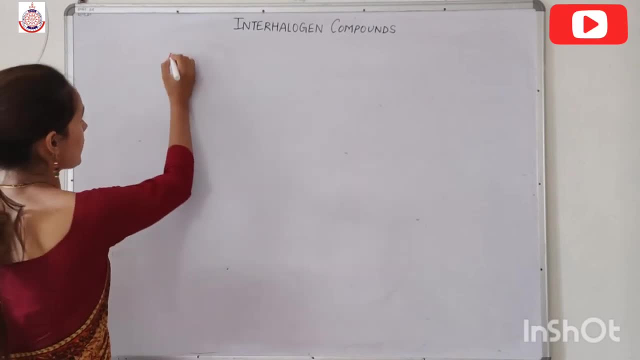 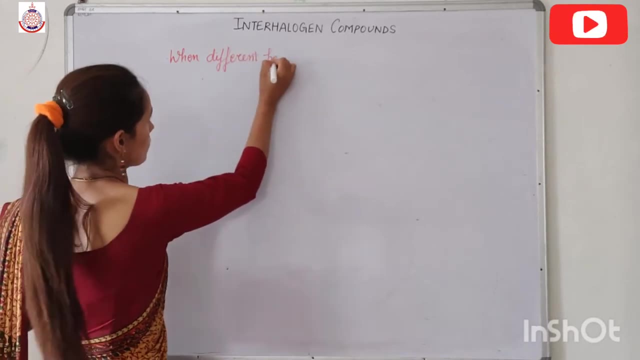 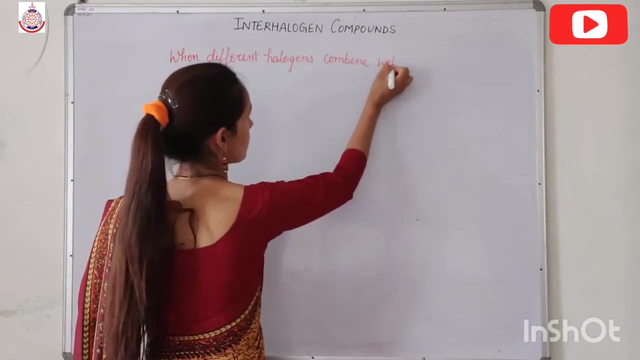 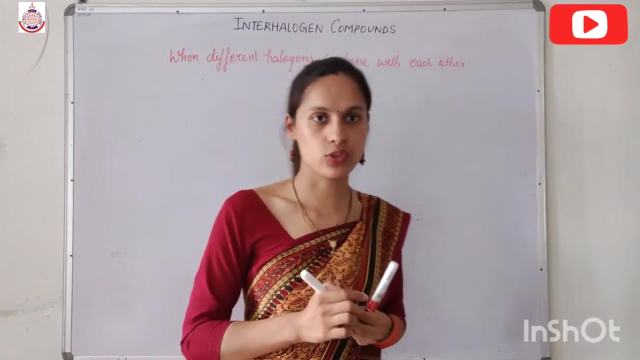 So the definition becomes: when different halogens, when different halogens combines with each other, when different halogens combine with each other, then we get interhalogen compounds, then we get interhalogen compounds. Now the interhalogen compounds, the general. formula of the interhalogens halogen compound. the general formula is XX-N. The general formula of different interhalogen compounds is XX-N where X, where this X represent the halogen of bigger size, the halogen of bigger size, or you may say the halogen of less electronegativity, and this represent the halogen. 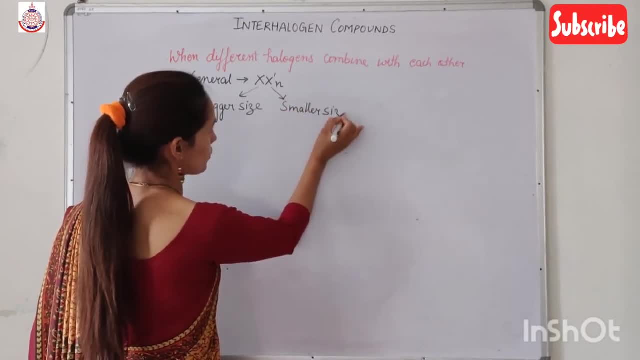 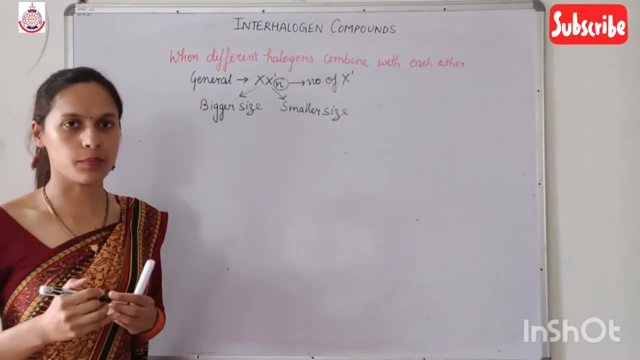 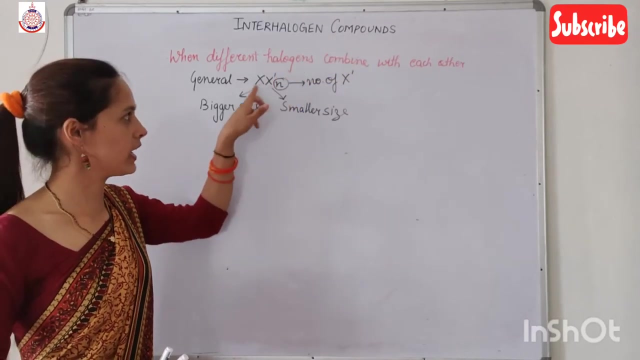 of smaller size or higher electronegativity, and this N represent the number of X dash. X represent the number of X dash, So interhalogen compounds. the general formula of interhalogen compounds is XX-N, where X represent the halogen of bigger size, X dash represent the halogen of. 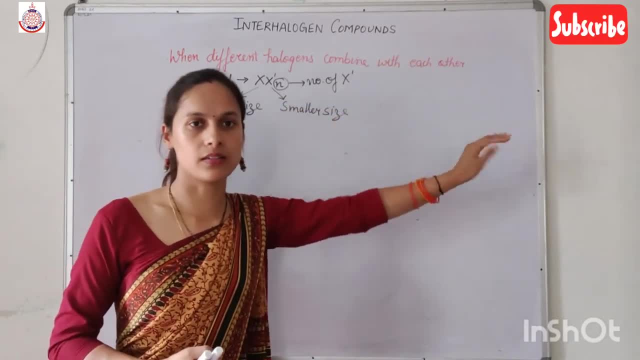 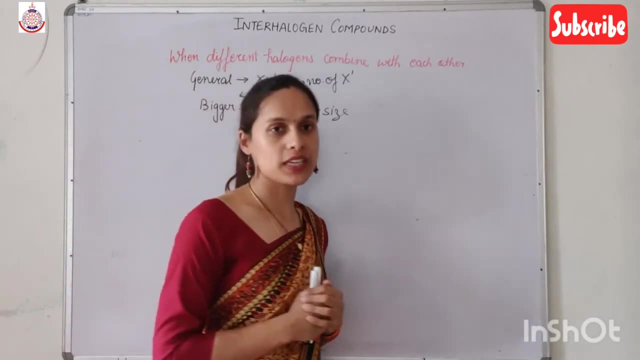 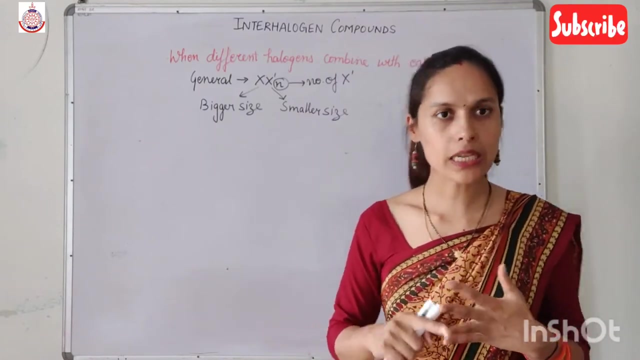 smaller size, and N represent the number of the halogen, which is smaller. Now in our previous videos we have studied that halogen shows four different positive oxidation state- plus 1,, plus 3,, plus 5 and plus 7- and on the basis of the oxidation state, 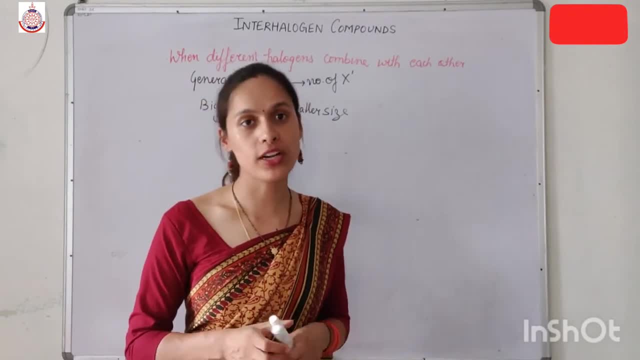 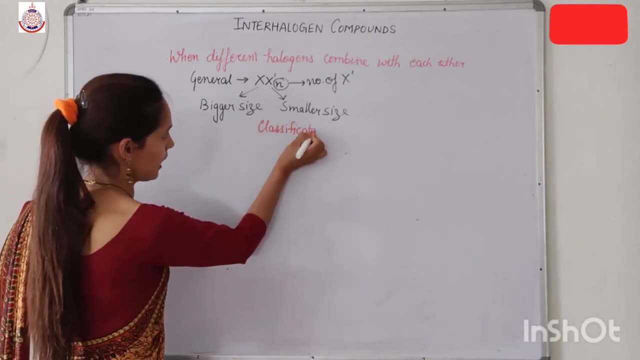 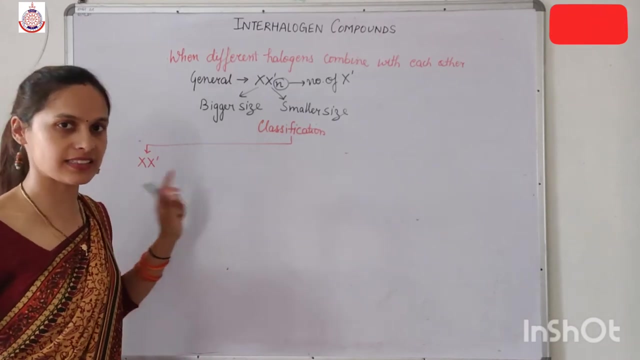 interhalogen compounds are classified into four different categories. So interhalogen compounds are classified into four different categories. Now, what are these four different categories? on the basis of plus 1 oxidation state, that is, XX dash. second, on the basis of plus 3 oxidation: 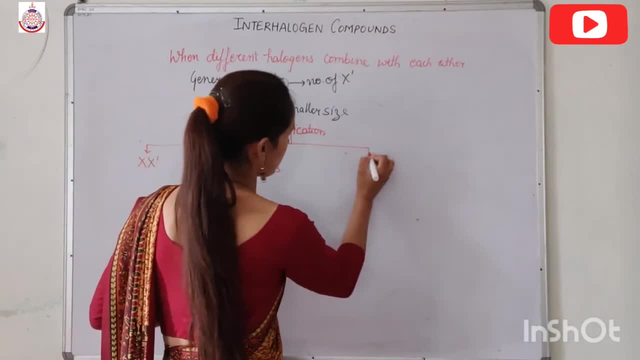 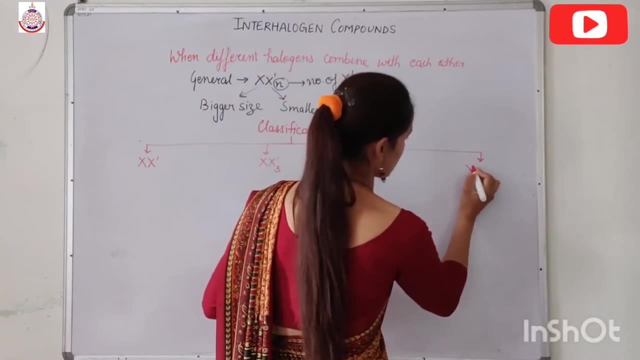 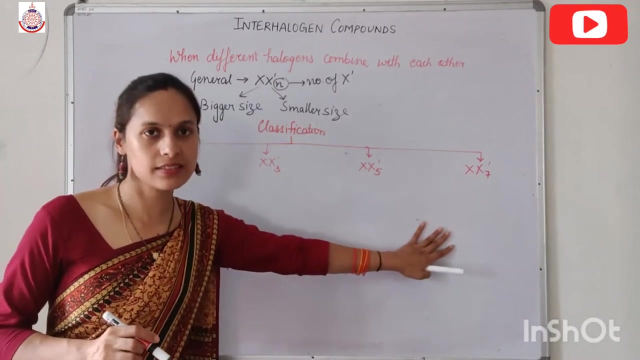 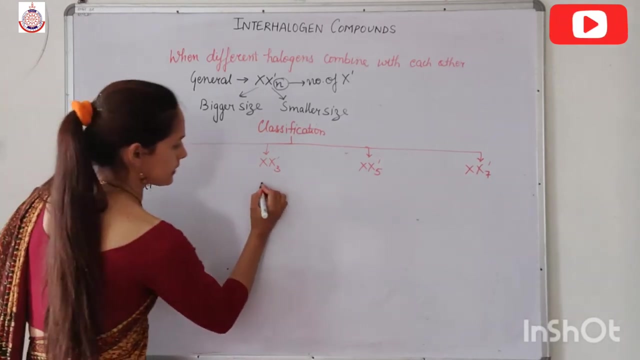 state, that is XX3 dash. third, on the basis of plus 5 oxidation state, that is XX5 dash. and fourth, on the basis of plus 7 oxidation state, that is XX7 dash. Now the different examples of these different interhalogen compounds are: first, we get ClF, ClF3 and ClF5, but we didn't get ClF7. 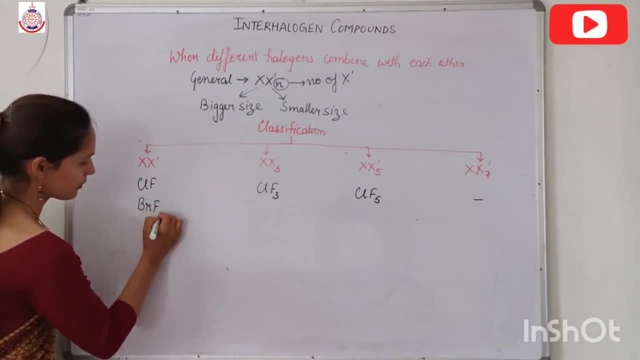 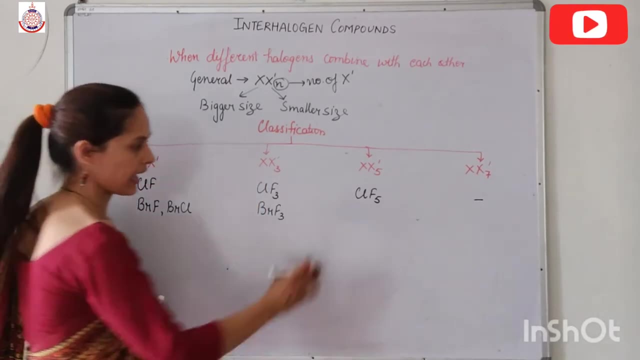 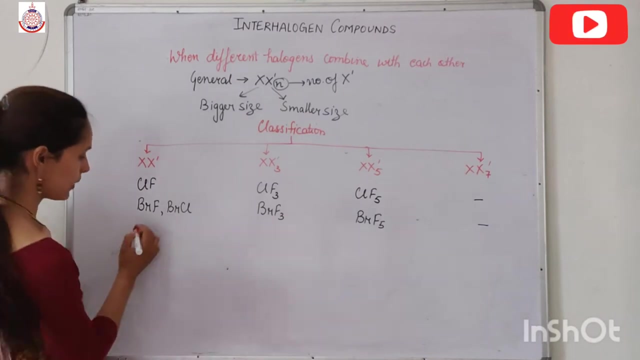 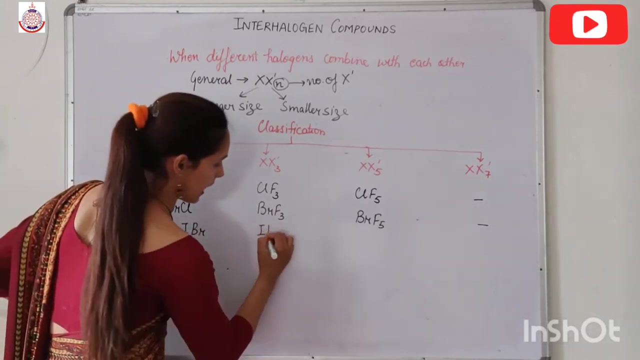 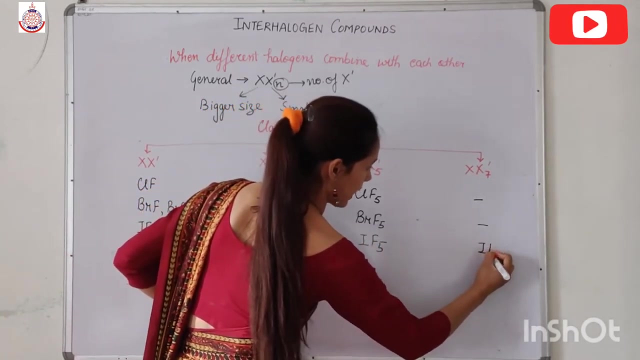 Next, we are getting BrF and BrCl, BrF3 and BrF5, but not BrF7.. We get IF, ICL, IBR, we get IF3, ICL3, we get IF5 and we also get IF7, we also get IF7. 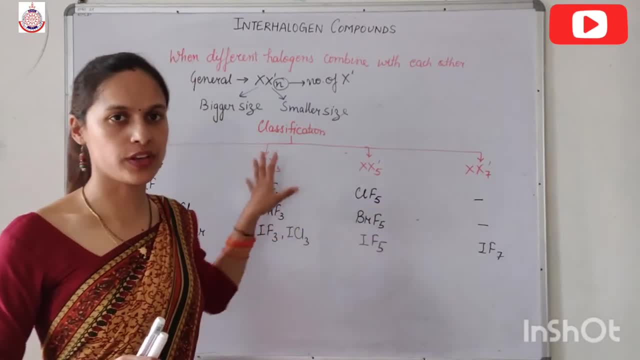 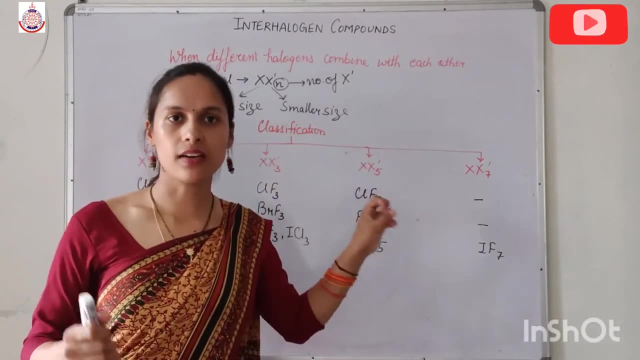 So these are the different examples which we get of different halogen, interhalogen types. Now, if we talk about the physical state of these different compounds, we get ICl, IBr, we get ICl3, we get ICl4, we get ICl5 and we also get ICl7. 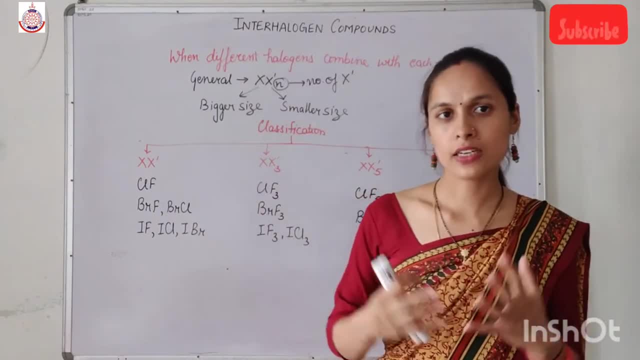 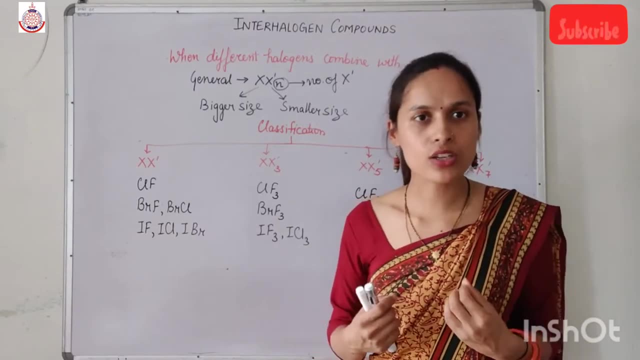 So these are the different examples which we get of different halogen, interhalogen types, As we know that with the increase in the size, with the increase in the atomic mass, what happens? The magnitude of the wonderful force of attraction increases and due to the 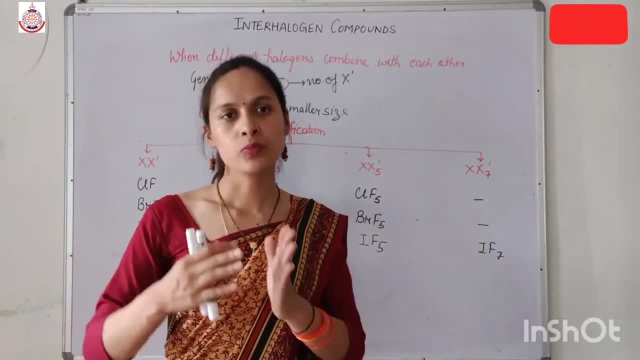 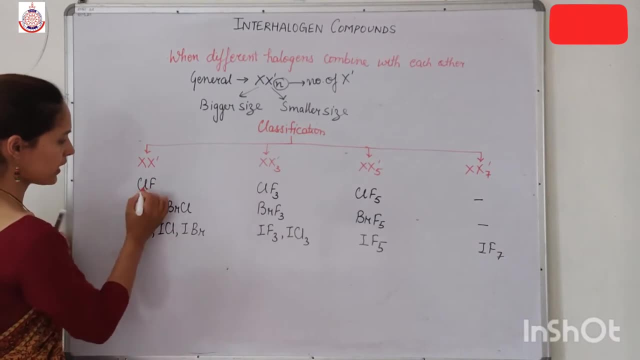 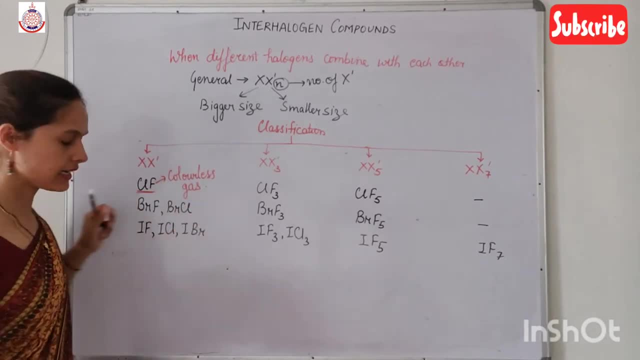 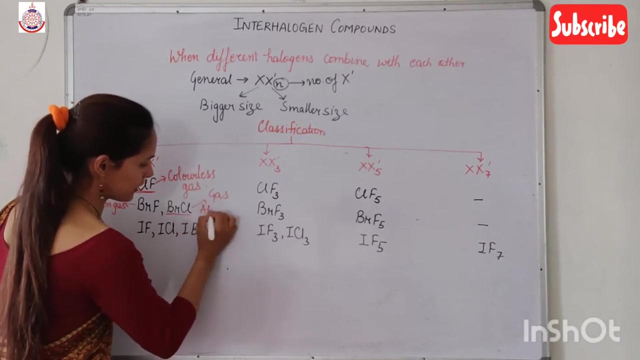 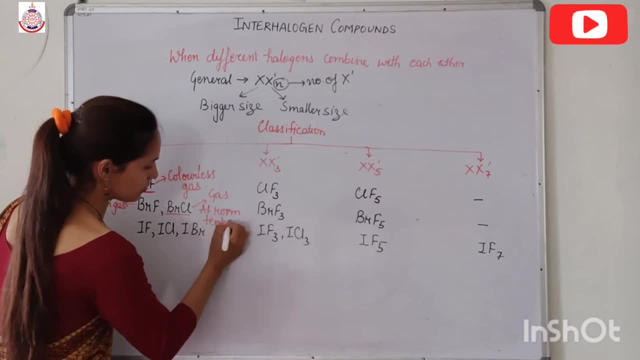 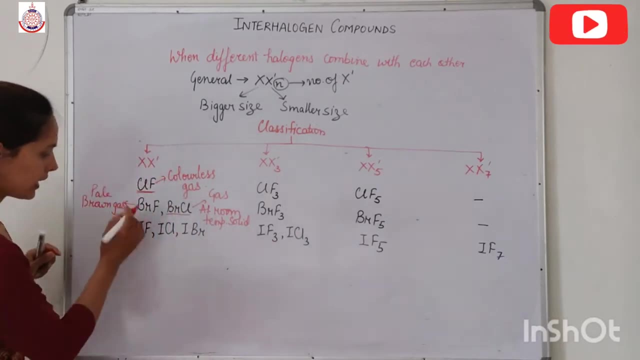 But at room temperature, we get this BrCl in the form of solid state. We get this BrCl in the form of the solid state. Now, if I talk about ClF, ClF is a tellerless gas. Now, if I talk about ClF, this ClF, this Clf is highly unstable. 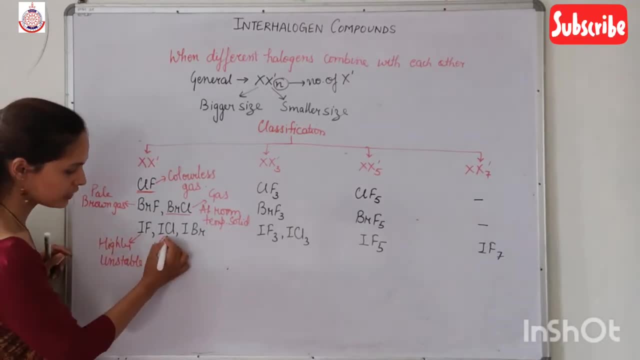 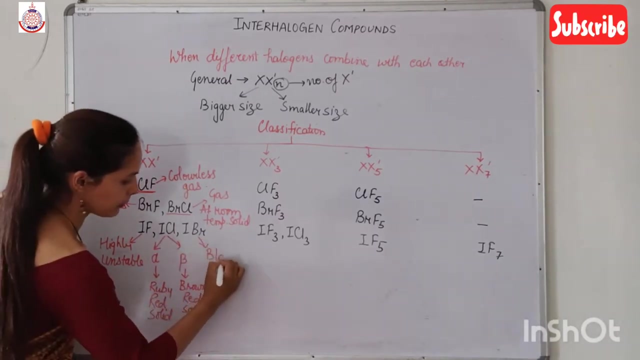 And if I talk about Clf, Clf exists in two forms: alpha form and beta form. Alpha form is a ruby red solid, It is a ruby red solid, and the beta form is the brown red solid- brown red solid. and if I talk about IBR, IBR is a black solid. So the first member of this family, that is. 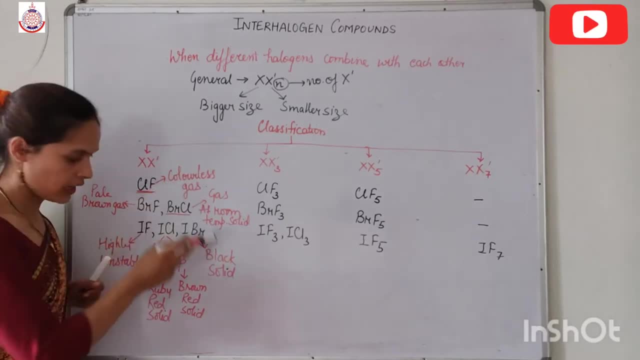 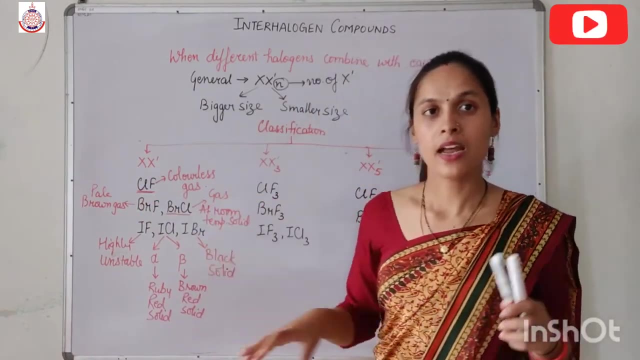 XX dash. the first member of this family is a colorless gas, while the last member is a black solid. Why? Because, as we move from CLF to IBR, what happens? The Wonderwall force of attraction increases. and due to the increase in the Wonderwall force of attraction, what? 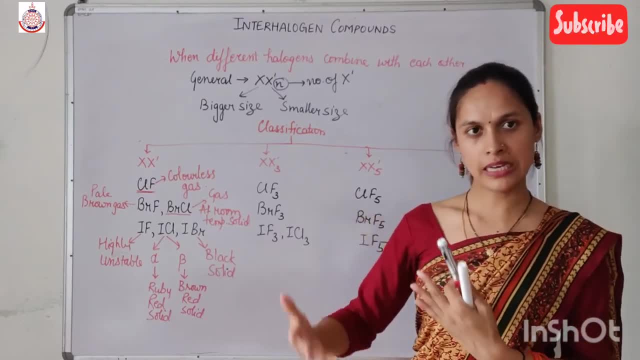 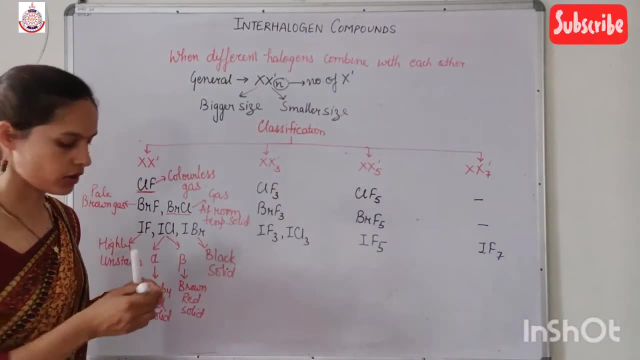 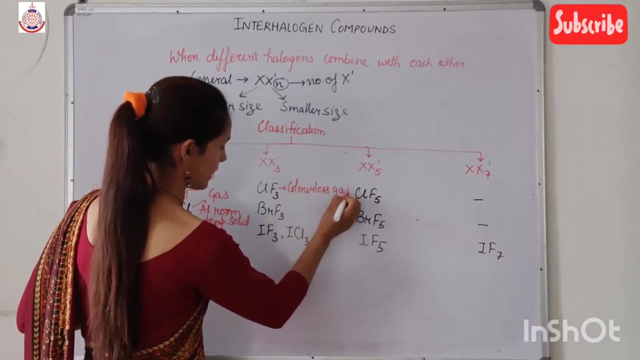 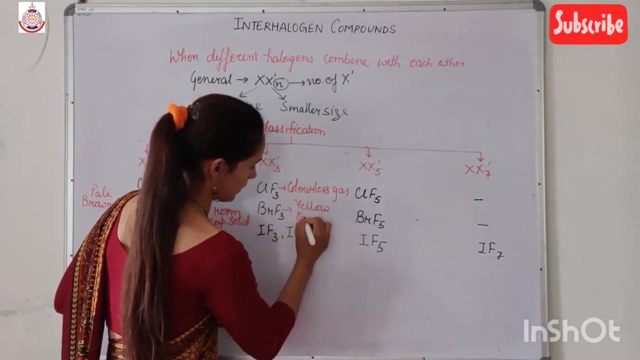 happens, The state becomes a liquid gas to liquid liquid to solid. Now, if I talk about XX3 dash, if I talk about XX3 dash, this CLF3 is a colorless gas. It is a colorless gas. This BRF3, this BRF3 is yellow orange liquid. It is yellow orange liquid. Now, this IF3. 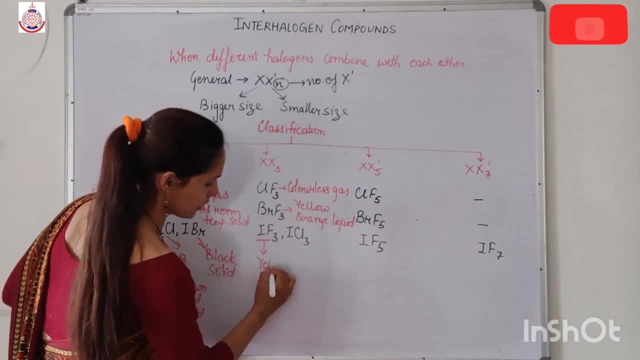 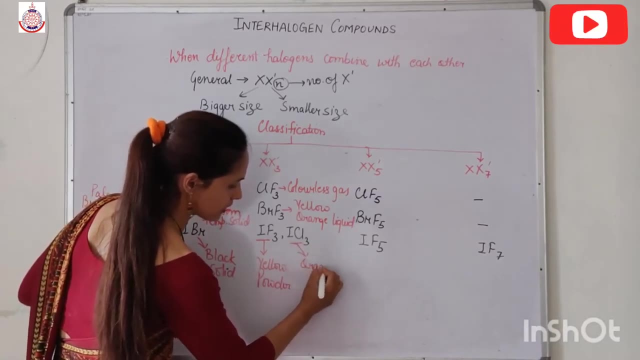 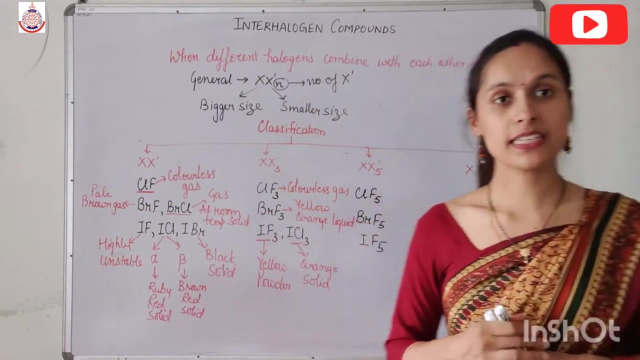 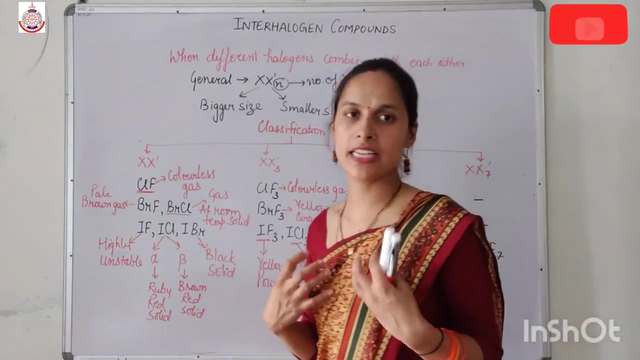 is yellow powder. It is a yellow powder And this ICL3 is orange, orange solid. In our previous videos also, we have studied that halogens are colored. halogens are colorful because they absorb the radiations in the visible light and the the remaining light. 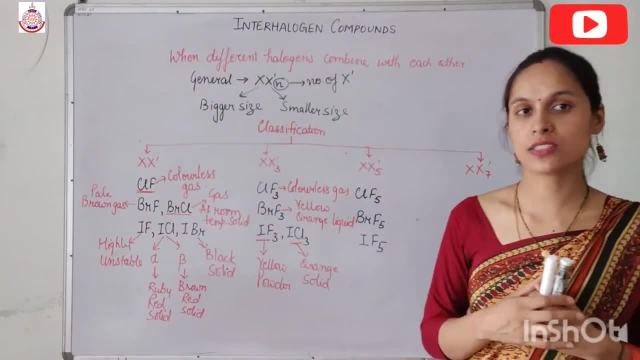 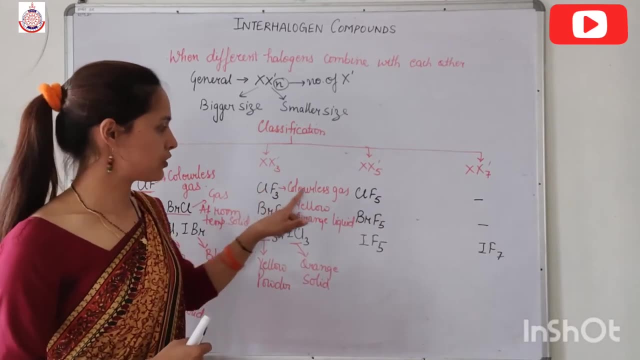 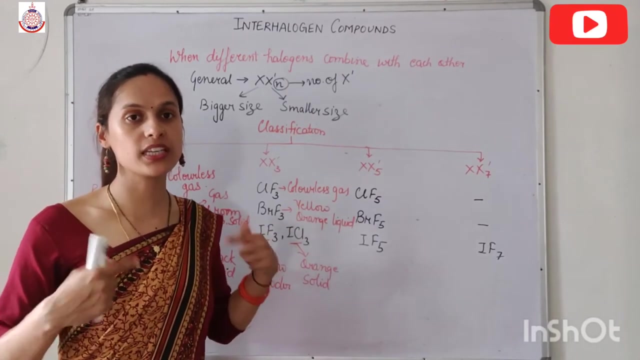 which they emit, that is, also comes under the visible reason as a result of which they become colored. So that's why we are getting different colors. So CLF3 is a colorless gas and ICL3 is orange solid. So again, gas can gas converted into solid due to the increase. 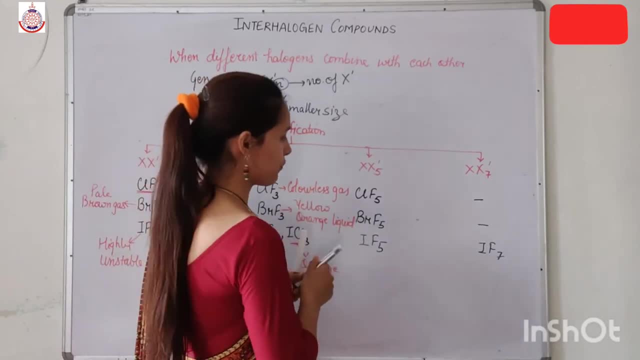 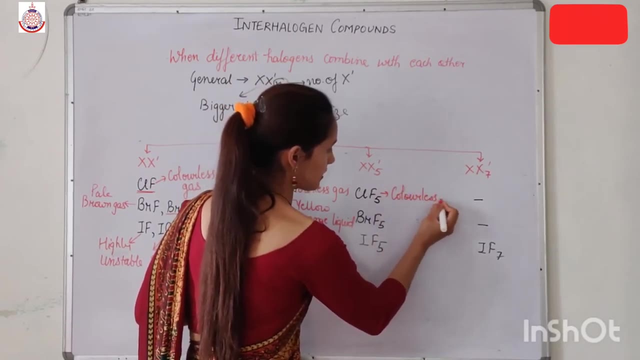 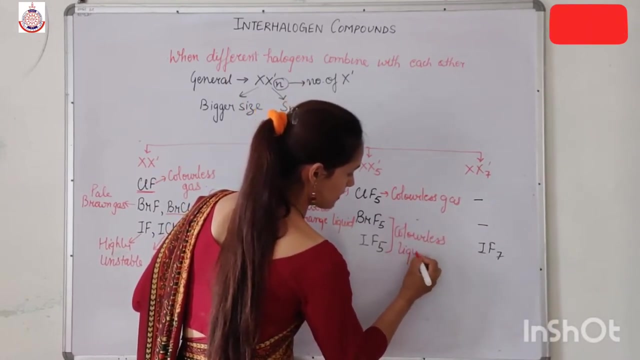 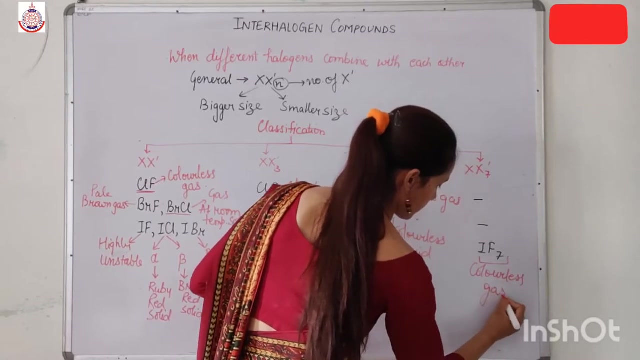 in the Wonderwall radii. Next, this CLF5,. this CLF5 is a colorless gas. It is a colorless gas and these two are colorless liquid. These two are colorless liquid and this one, this IF7, is a colorless gas. This IF7 is a colorless gas. So these are the different physical 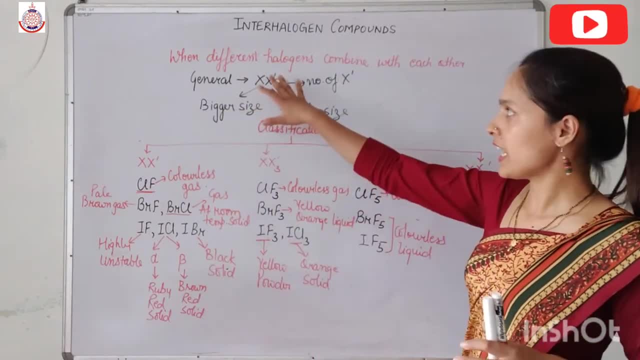 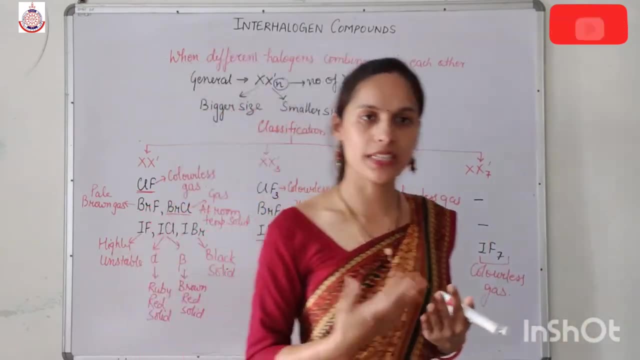 states of the different interhalogen compounds. So interhalogen compounds are the compounds which are formed by the different halogens. When different halogens combines together, then they form interhalogen compounds. The general formula of the different interhalogen compound is X6-N, where X represent the halogen. 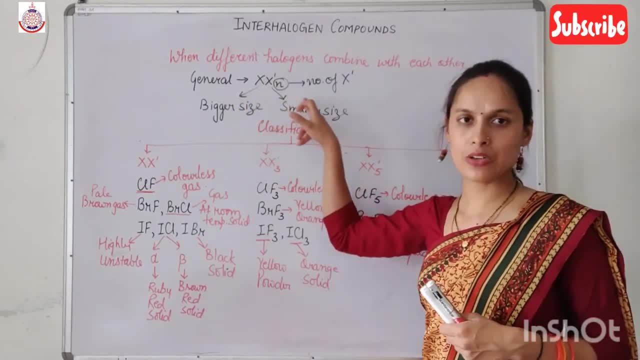 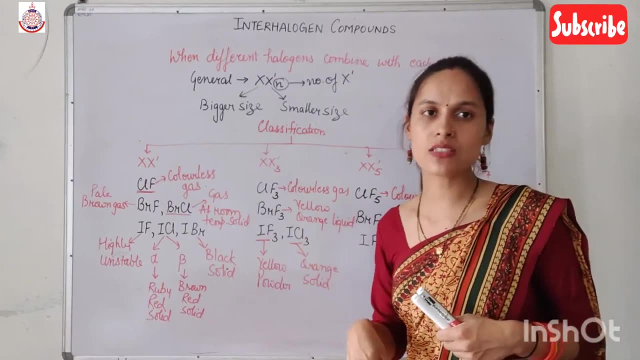 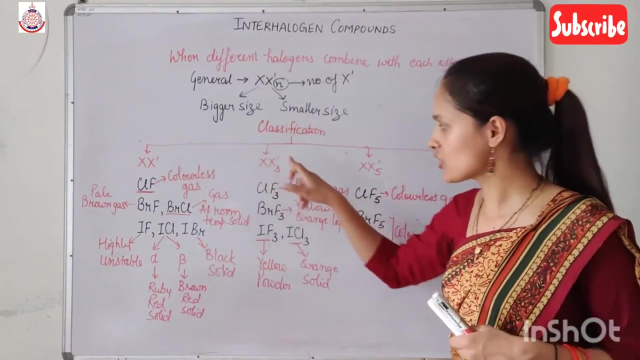 of bigger size. X- dash represent the halogen of the smaller size and N represent the number of the halogen of smaller size. Now, depending upon the oxidation state exhibited by the halogens, the interhalogen compounds are classified into four categories: XX dash, XX3 dash. 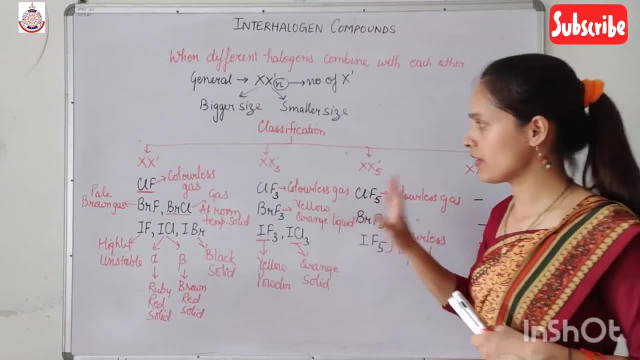 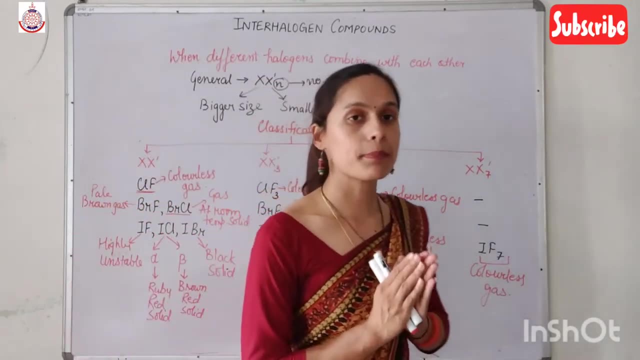 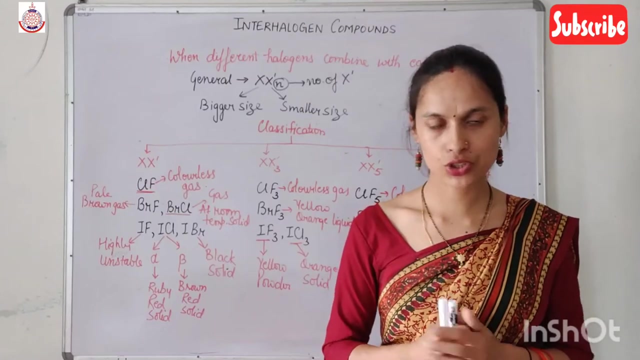 XX5 dash and XX7 dash. And these are the different examples of the different halogens. Now, if we talk about the preparation of the interhalogen compounds, so interhalogen compounds are prepared either by the direct combinations of the halogen or by the action. 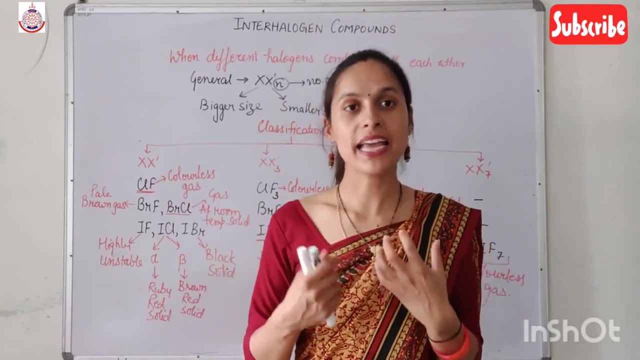 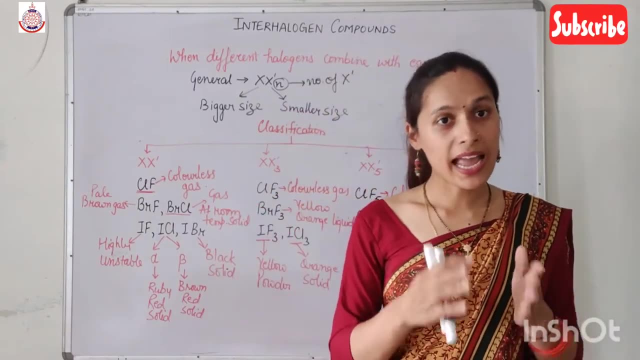 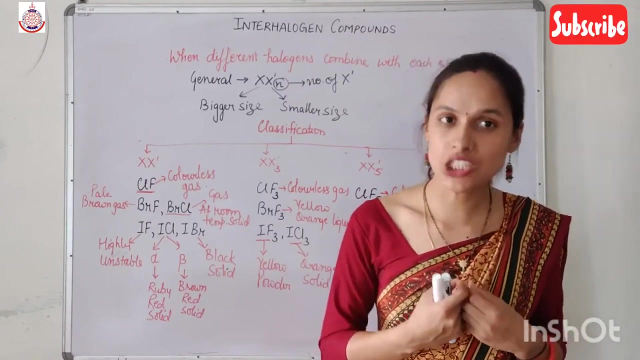 of a more electronegative by the action of a more electronegative halogens to the less electronegative interhalogen compound And the product. when different reactions take place, the product depend upon the conditions also. So while preparing we can prepare the interhalogen compounds, either by the direct combination or by the action of the lower interhalogen compounds to higher electronegative halogen. But depending upon the conditions we get different product. So now we will see the preparation of the interhalogen compounds. 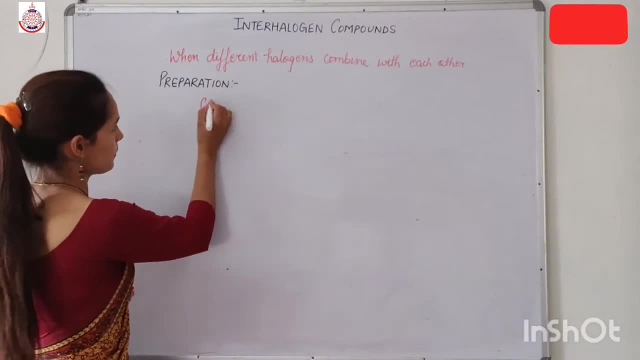 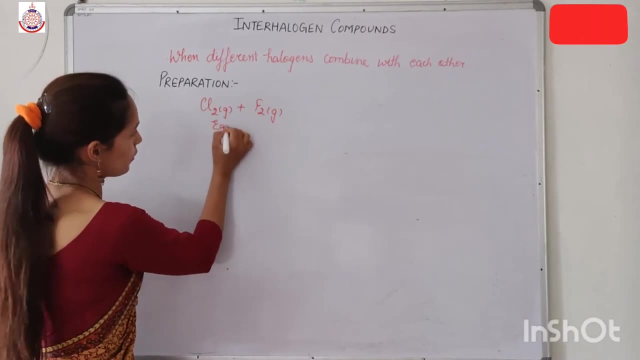 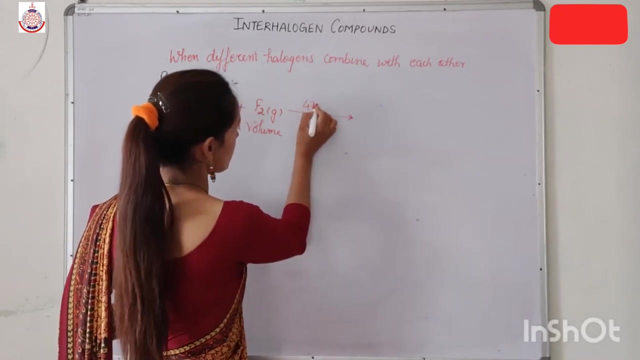 So in preparation, suppose Cl, Cl2 gas Reacts with F2 gas. Now if I take equal volume of chlorine and fluorine, if I take equal volume of chlorine and fluorine and keep the temperature- 473 Kelvin, keep the? temperature 473 Kelvin, then I get chlorine fluoride. then I get chlorine fluoride. And if I take F2 in excess, if I take F2 in excess and keep the temperature 573 Kelvin, then I get ClF3,, then I get ClF3.. And if I react ClF gas with the F2 gas, if I react ClF gas, with the F2 gas at 475 to 575 Kelvin. then I get ClF3. So we can prepare the interhalogen compounds either by the direct combination or by the action of a more electronegative halogen. But if we change the condition, here I am taking equal volume, here I am taking. 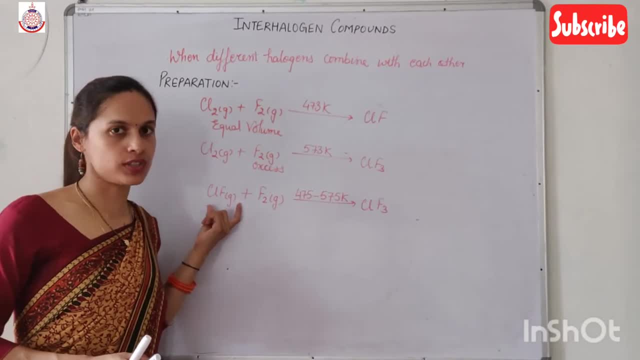 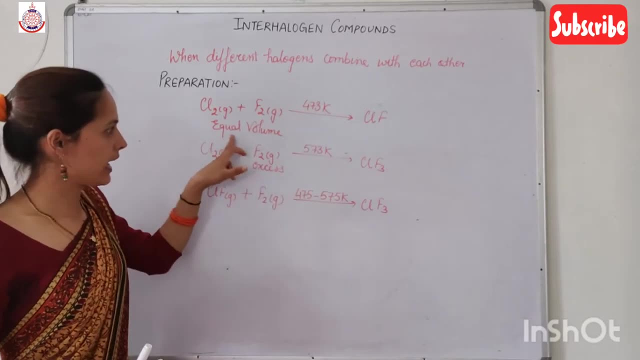 excess of fluorine. here I am keeping the temperature 473 Kelvin, here I am keeping the temperature 573 Kelvin. So by changing the temperature, by changing the conditions, the product also gets changed. So we can prepare interhalogen compounds, either by the direct combination or by the action of the lower halogen with the more electronegative halogen. We can prepare interhalogen compounds, either by the direct reaction or by the action of the more electronegative halogen to the lower interhalogen compounds to the lower interhalogen. 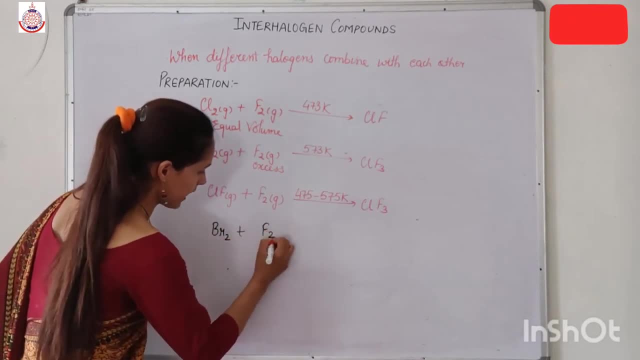 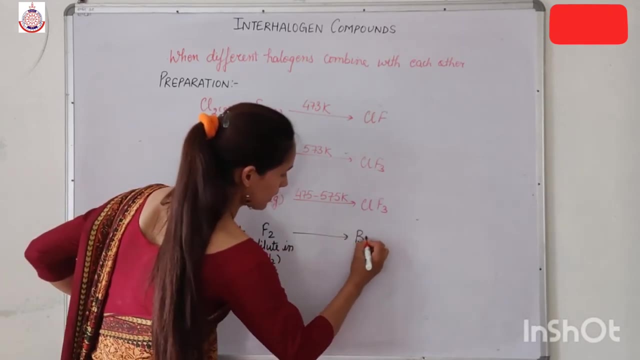 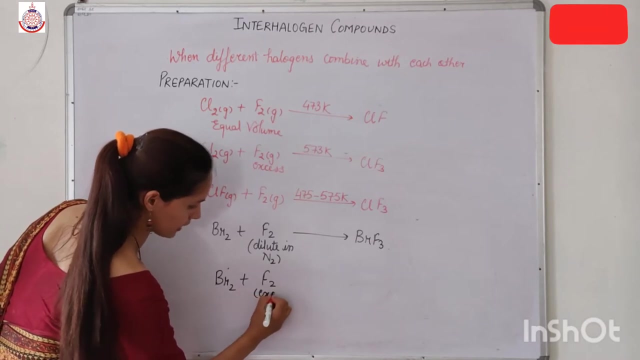 compounds. Br2 reacts with fluorine and that fluorine, if diluted in, diluted in N2, then I get BrF3. And Br2, when react with excess fluorine. when react with excess fluorine, then I get BrF2, when react with excess of normal fluorine. excess of normal fluorine. 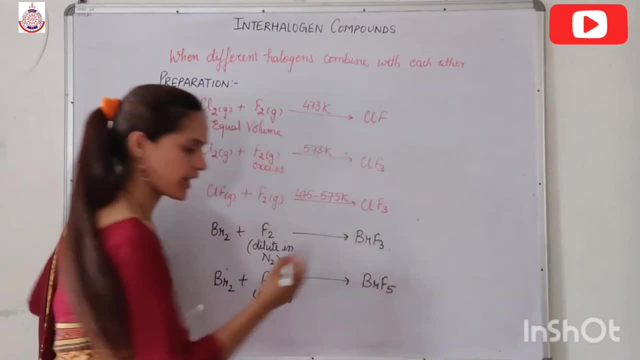 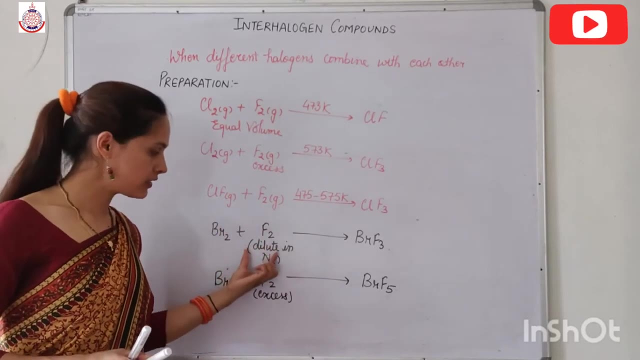 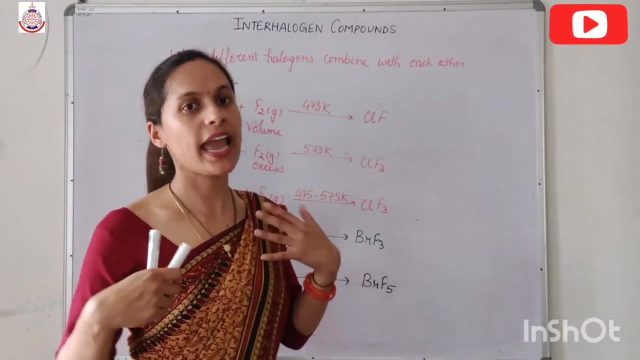 then I get BrF5. So in both the case, in both the case the reactants are only bromine and fluorine, But in first I have diluted fluorine in liquid nitrogen and in second I am keeping the fluorine in excess quantity. So due to the change in the condition, what happen? 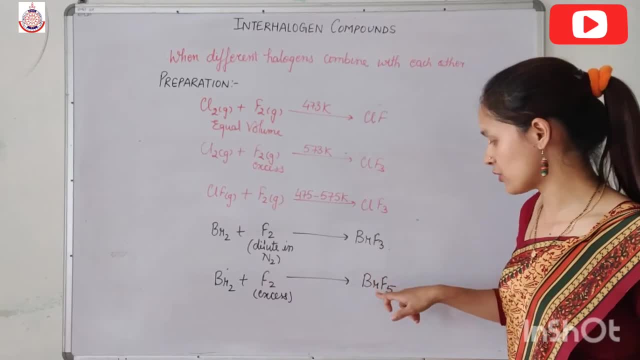 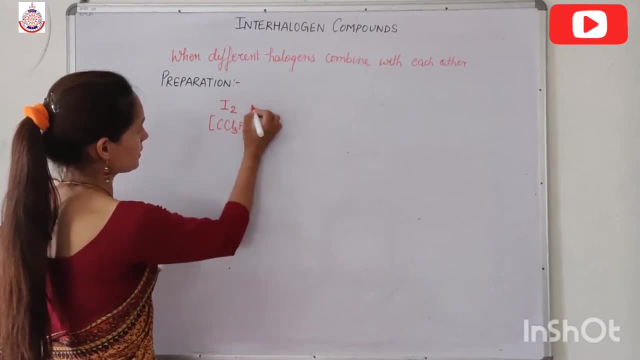 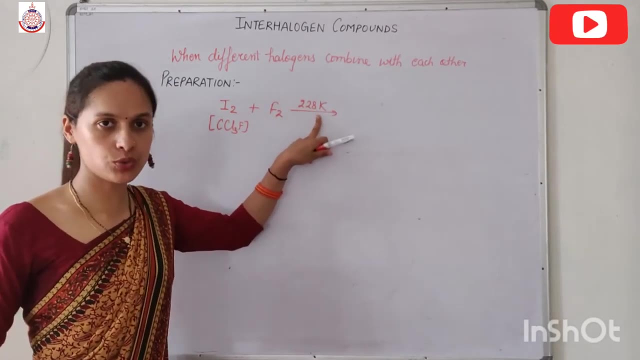 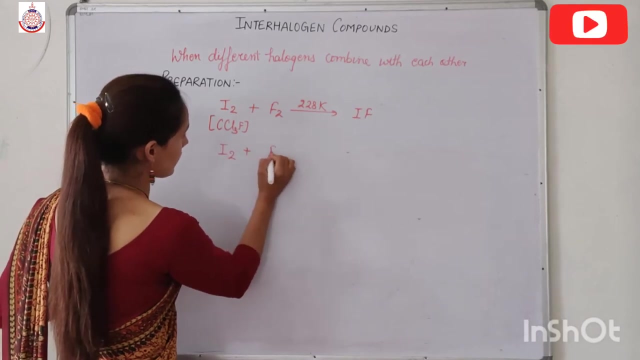 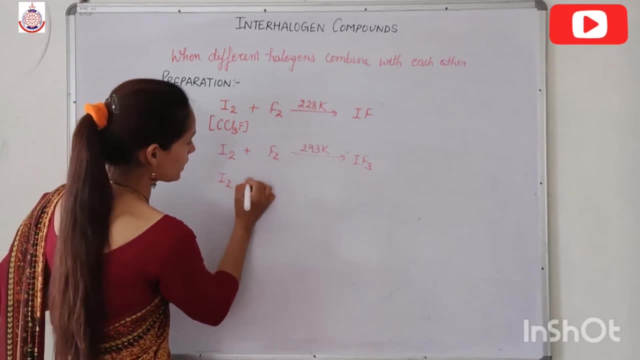 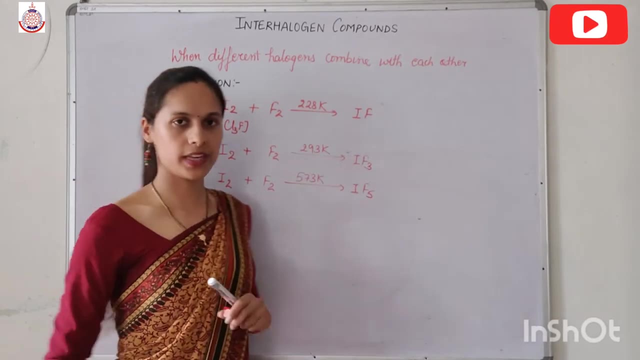 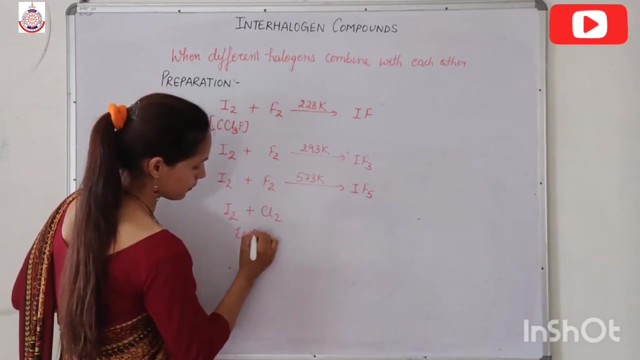 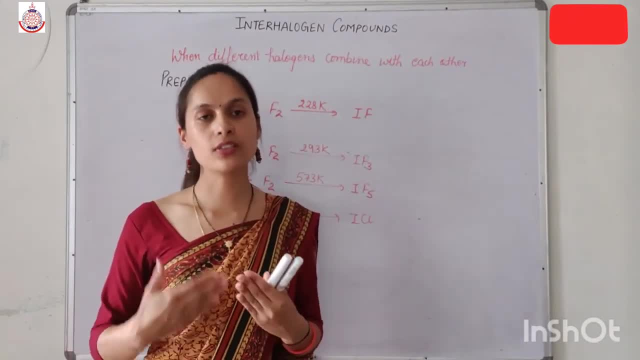 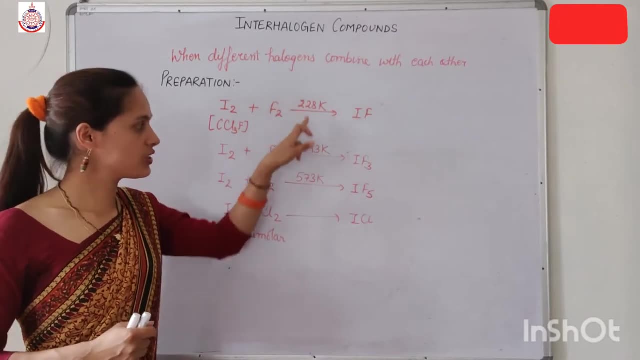 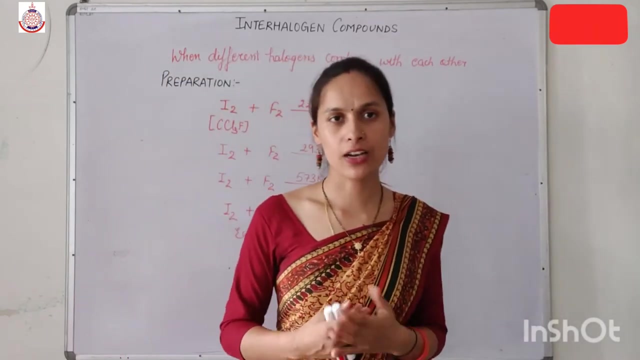 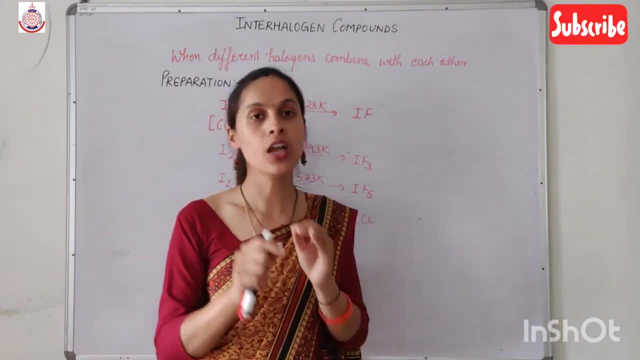 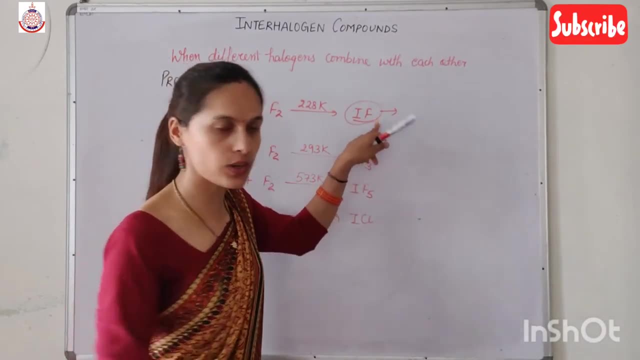 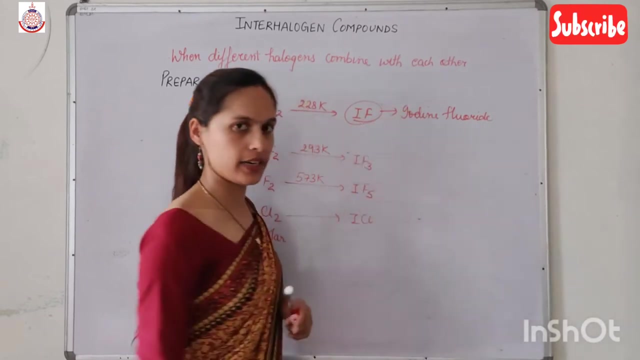 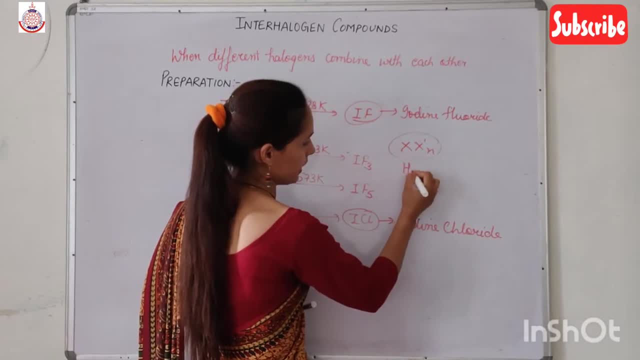 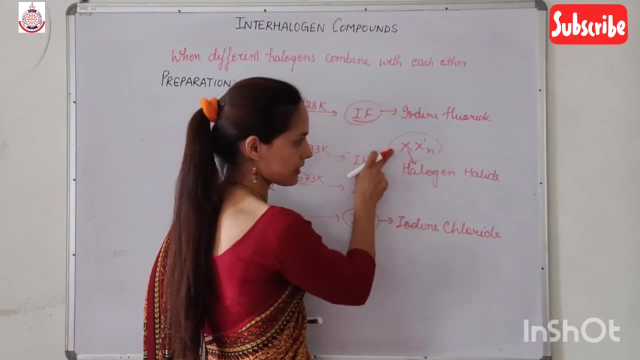 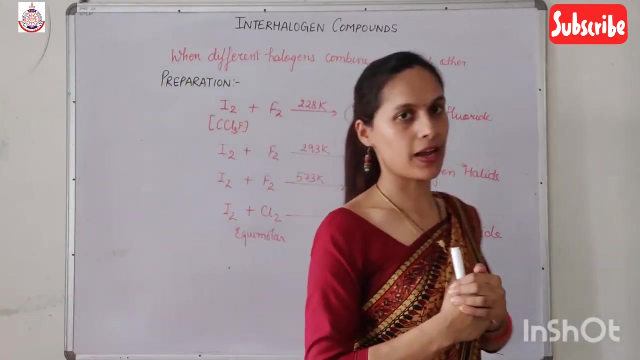 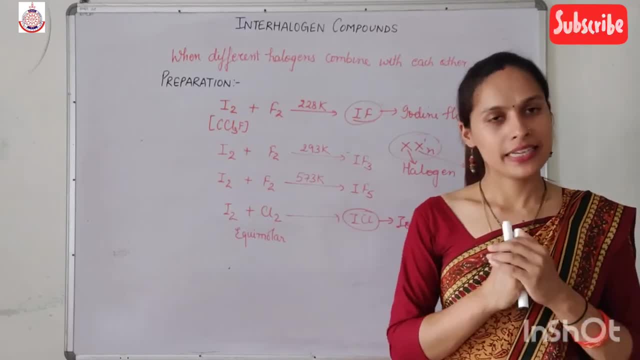 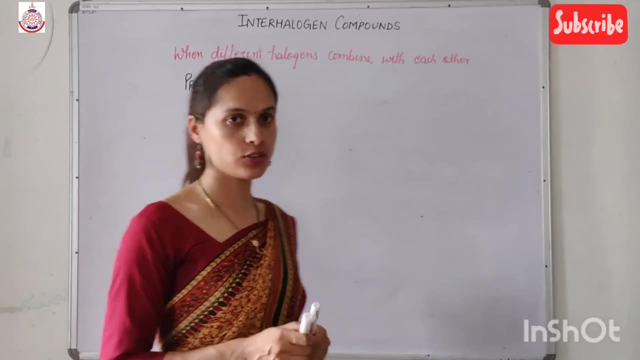 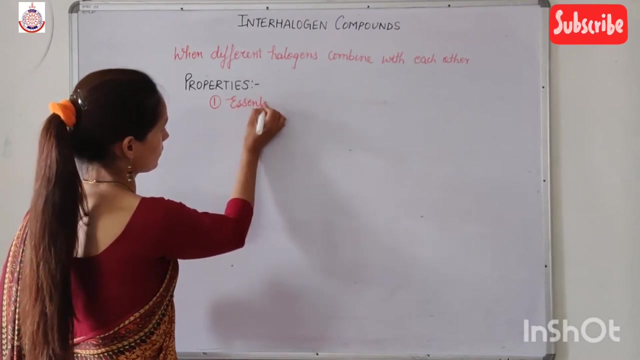 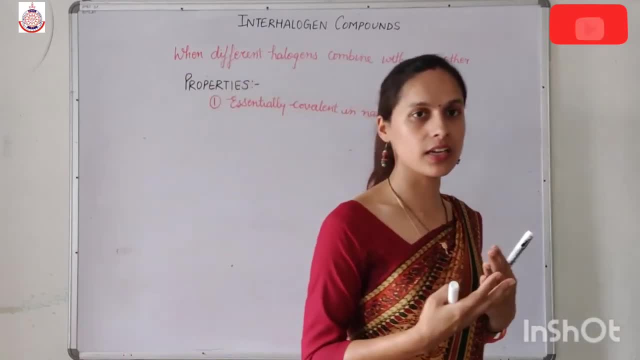 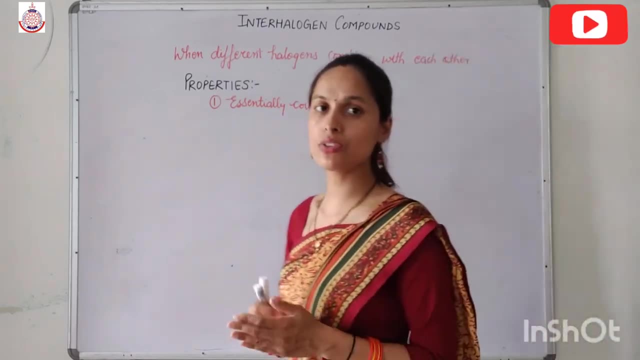 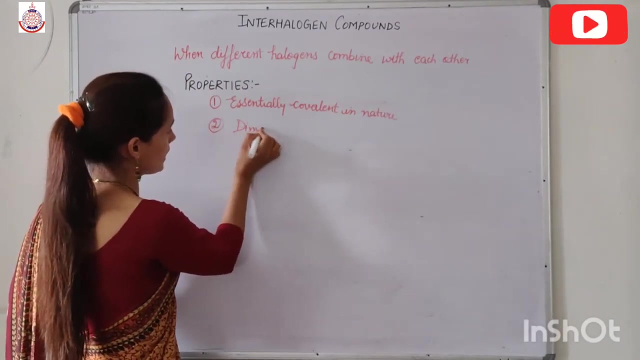 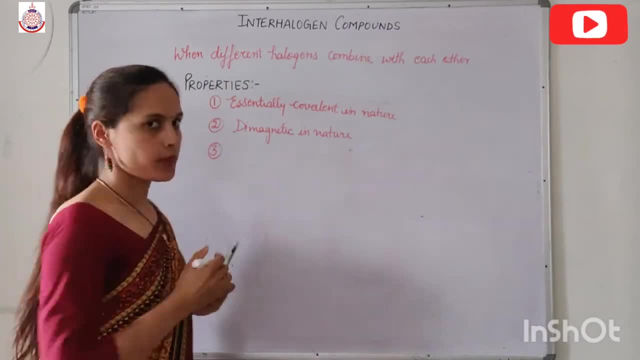 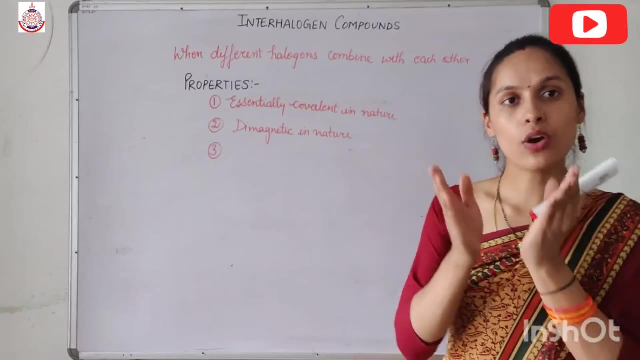 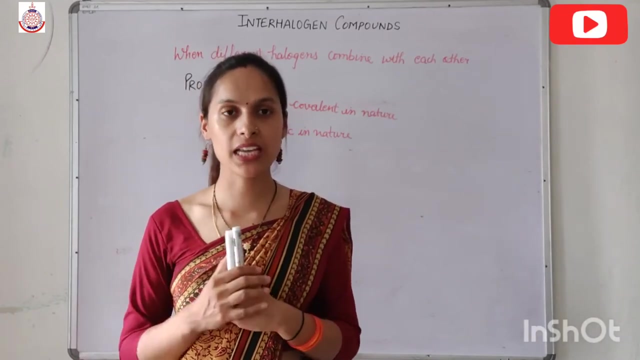 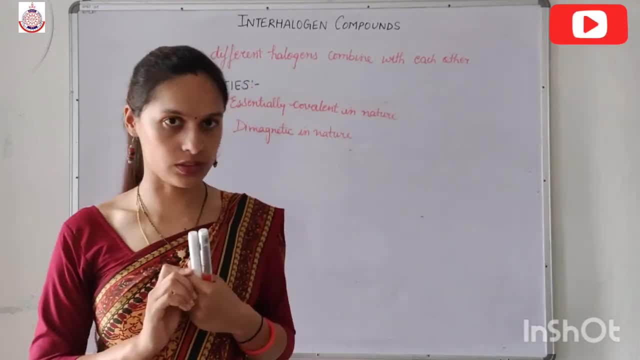 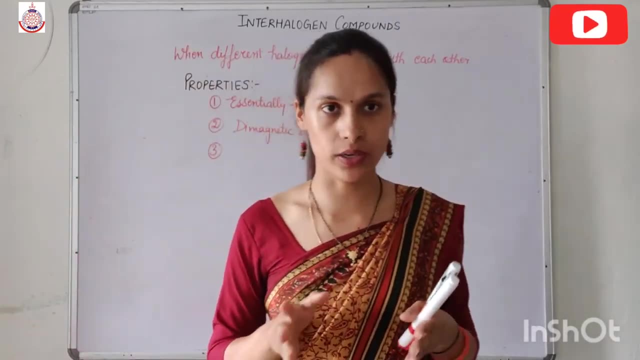 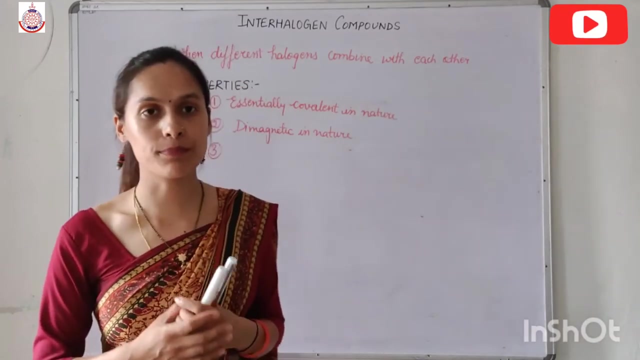 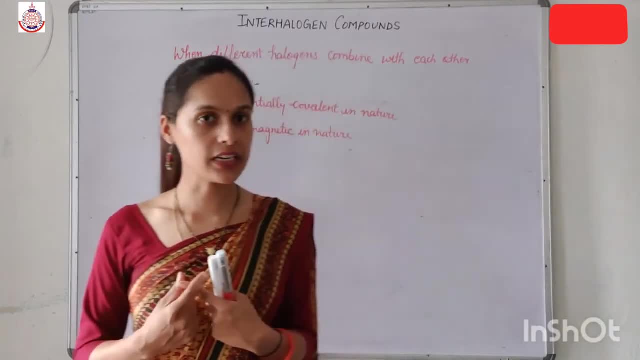 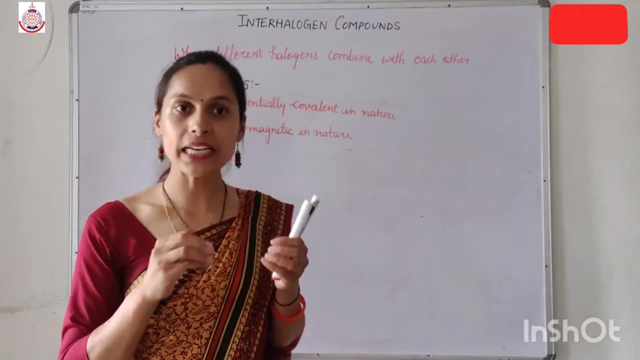 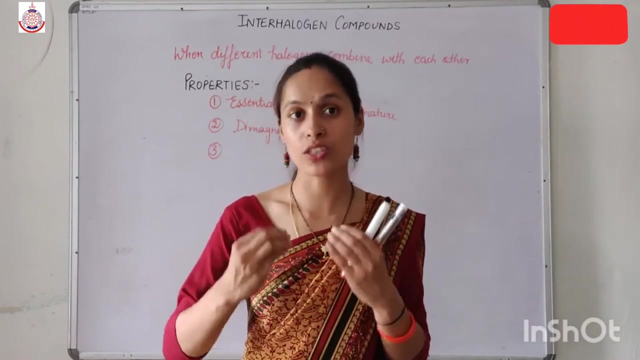 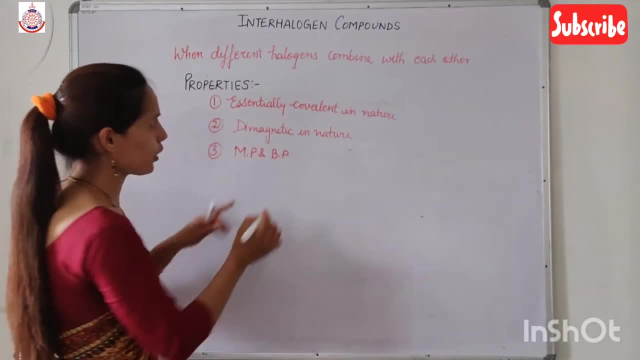 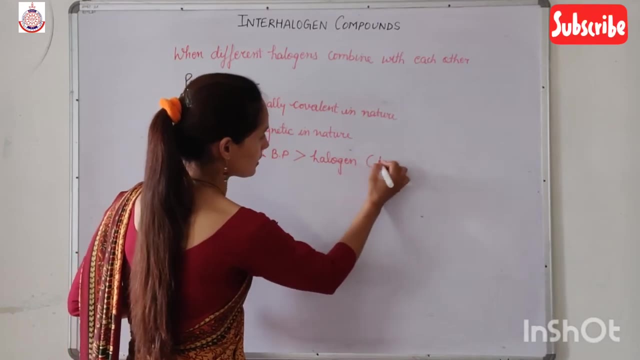 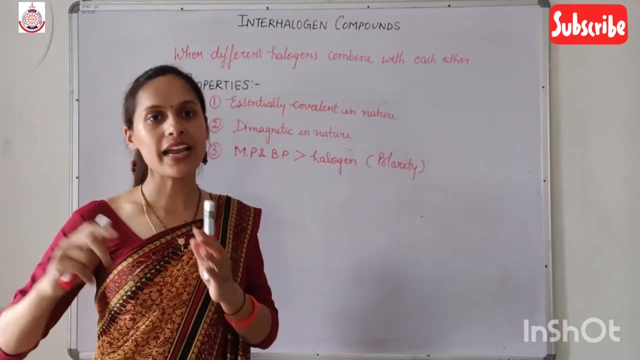 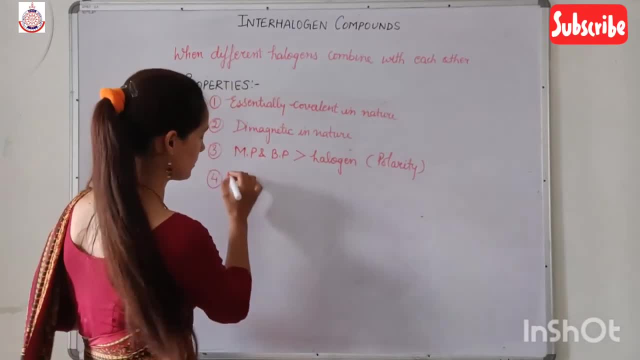 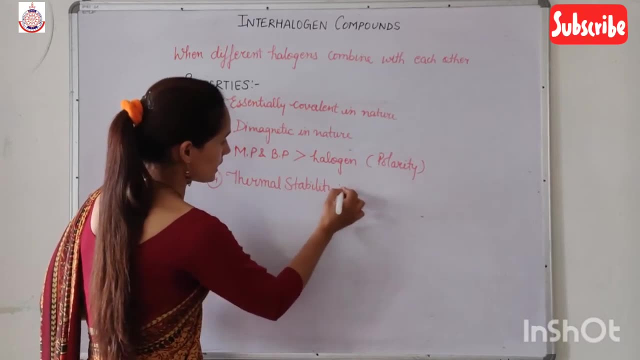 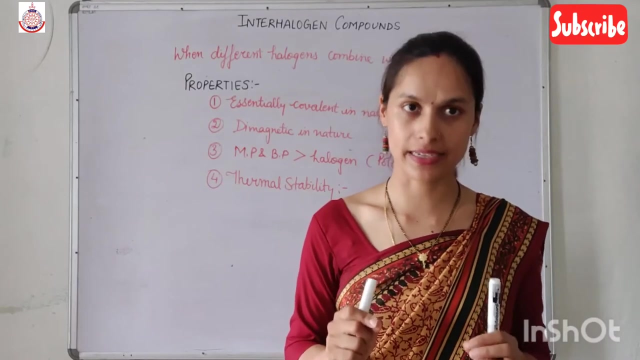 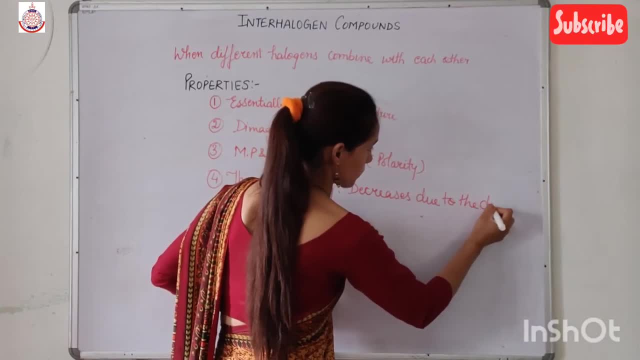 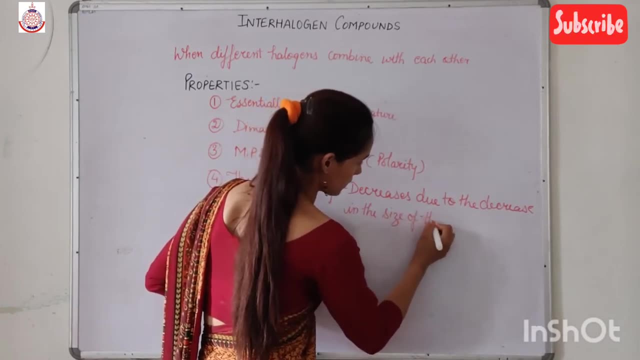 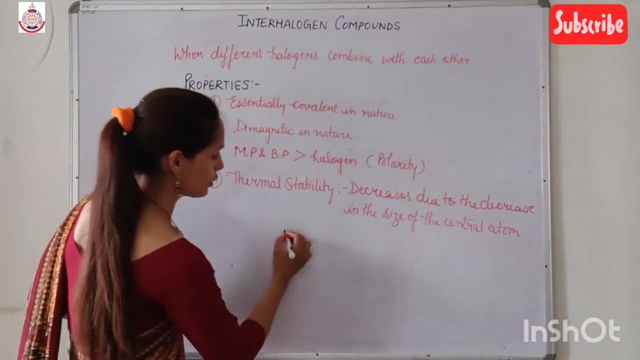 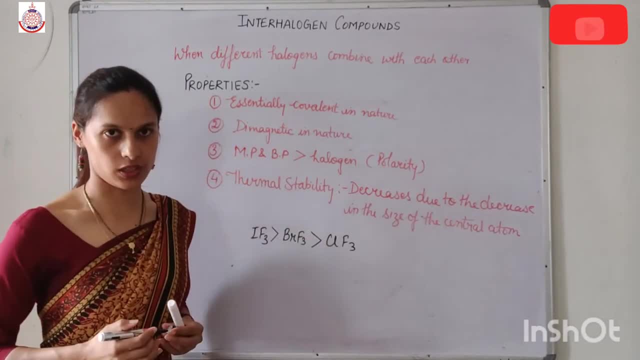 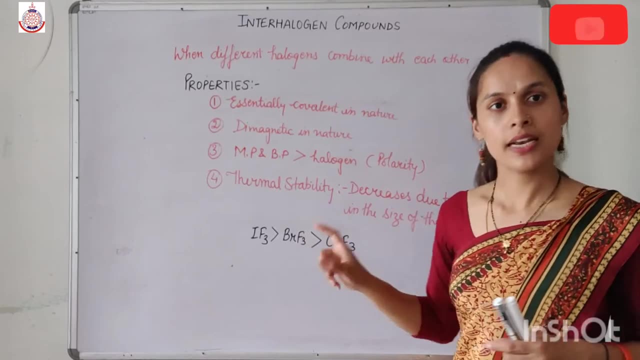 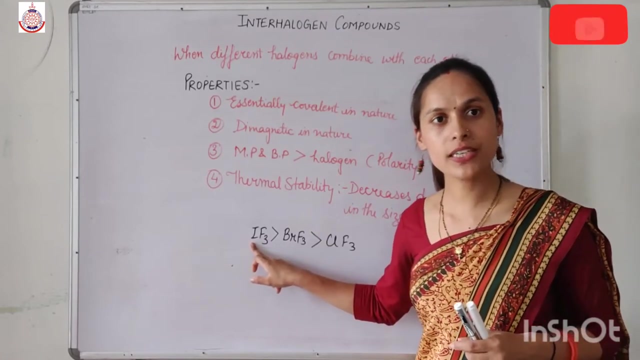 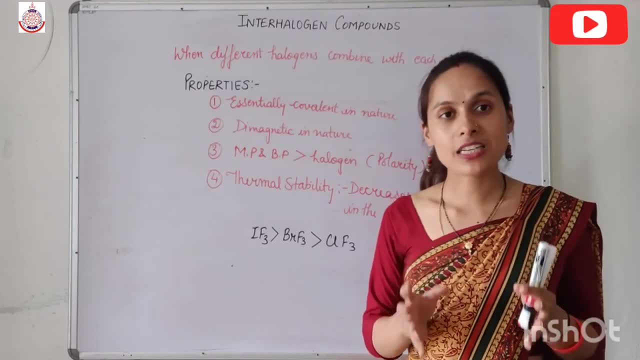 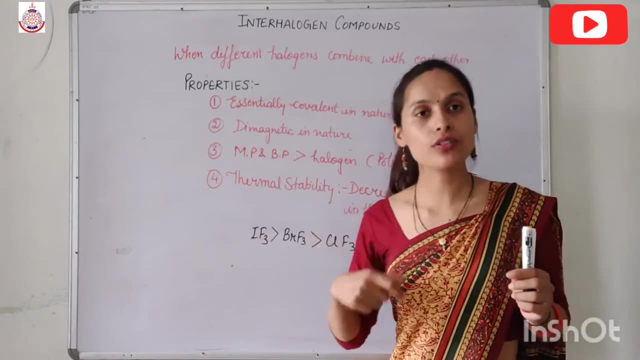 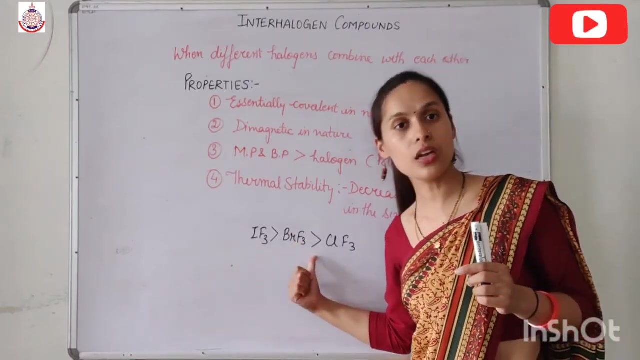 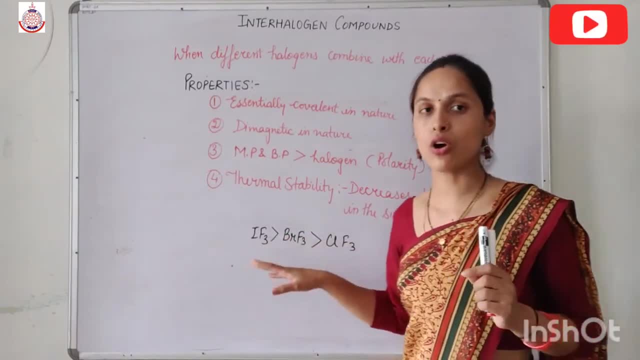 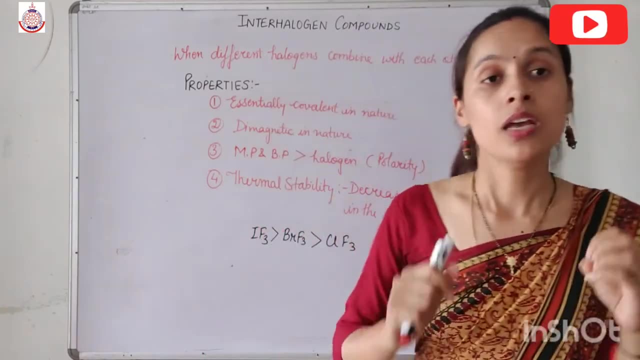 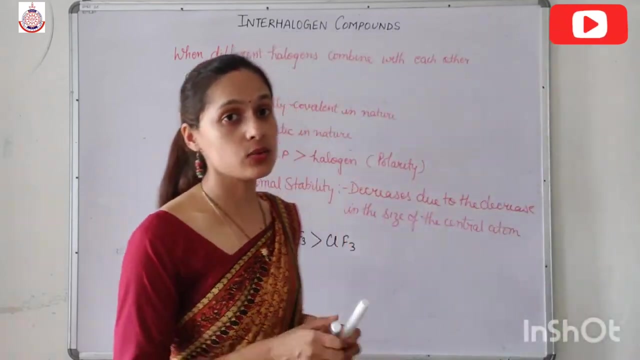 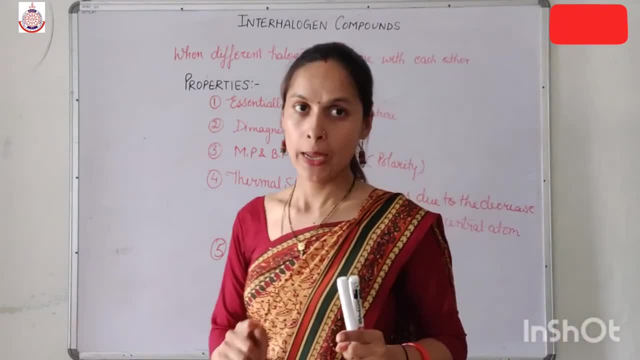 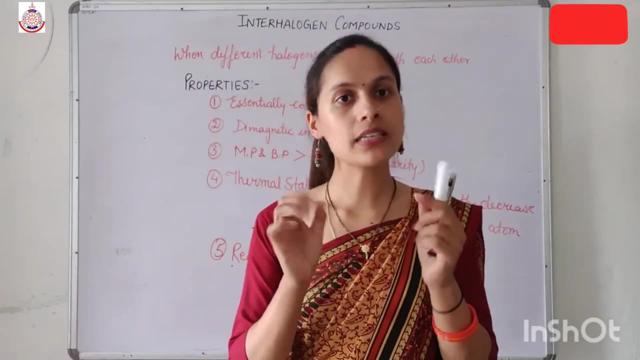 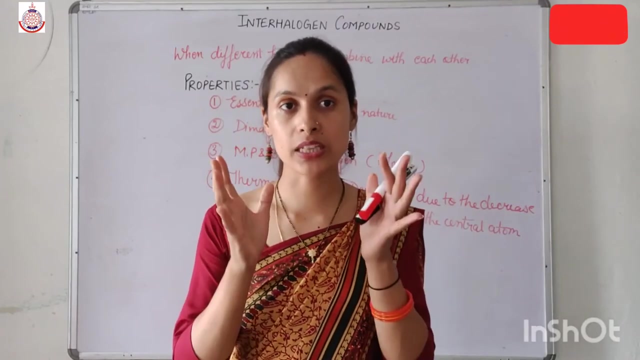 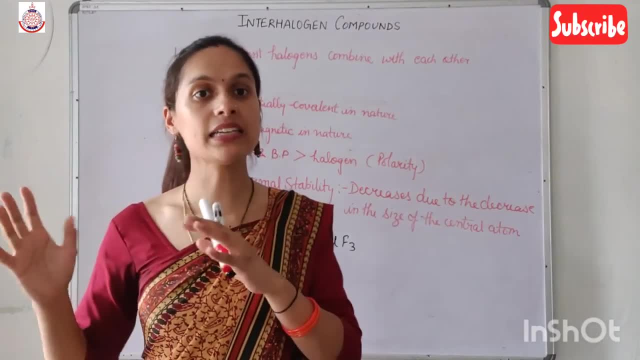 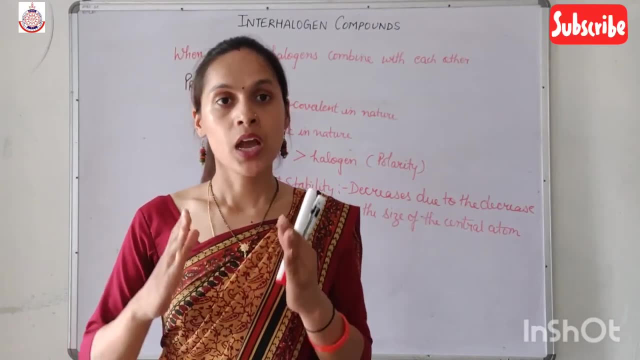 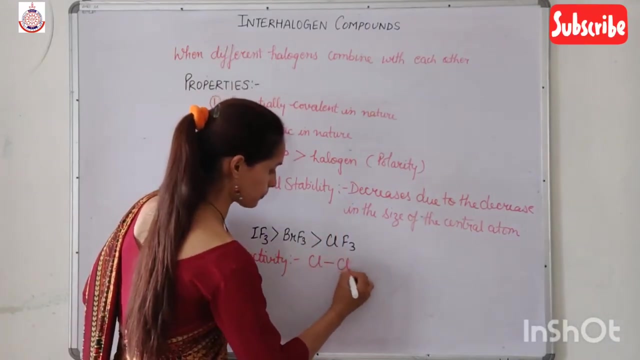 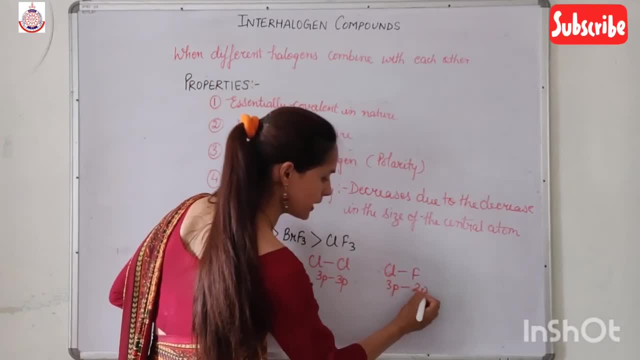 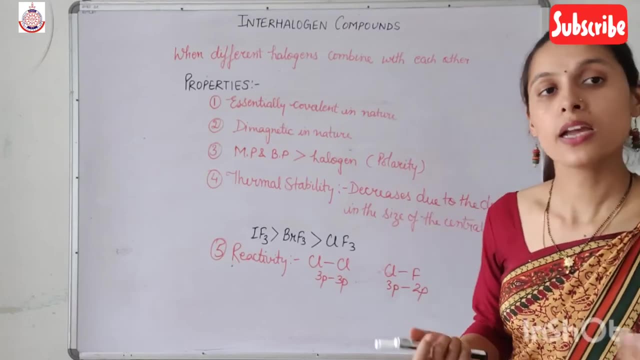 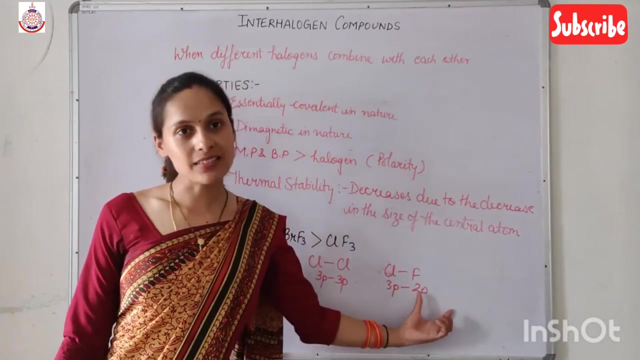 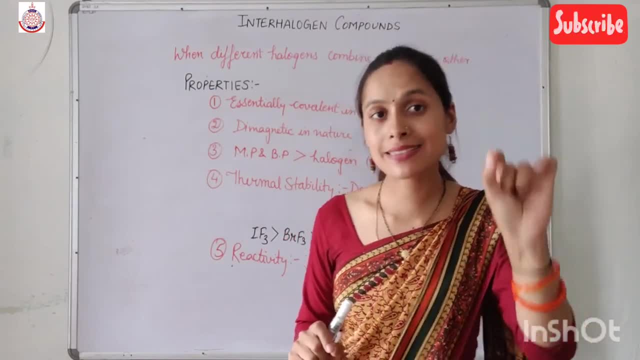 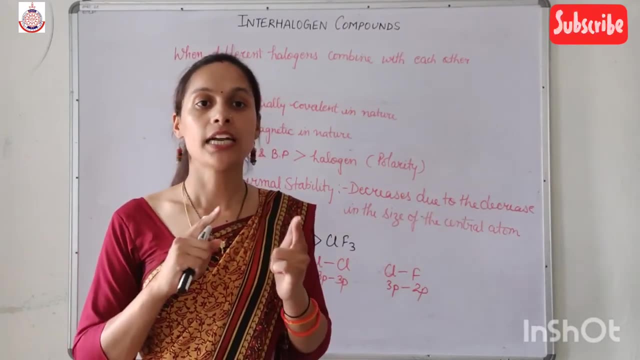 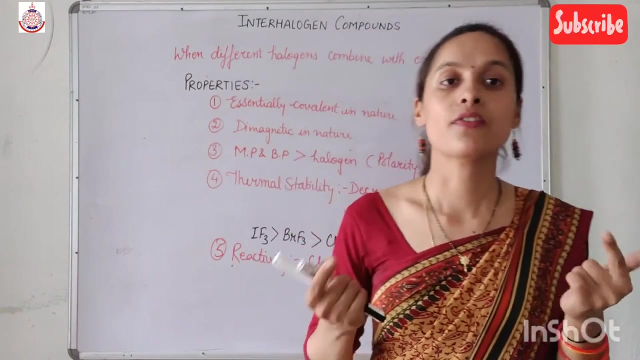 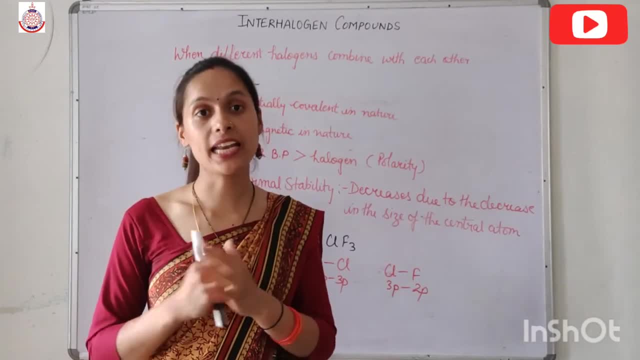 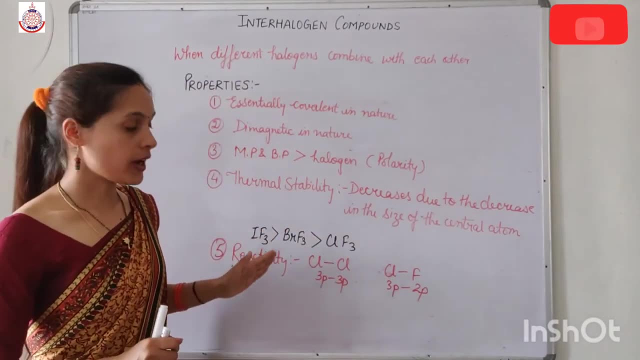 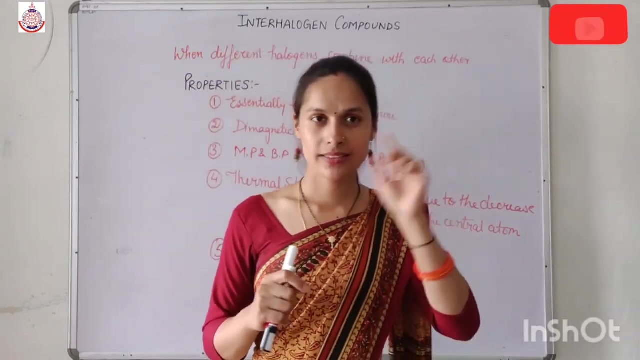 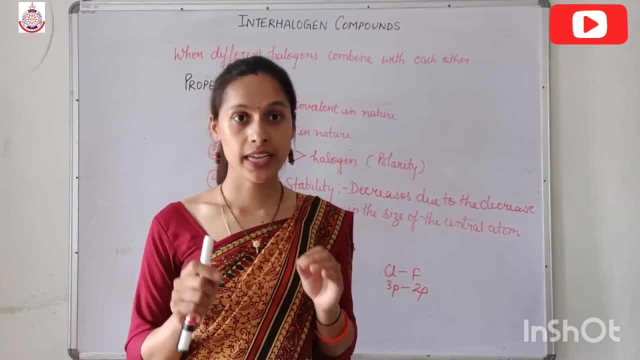 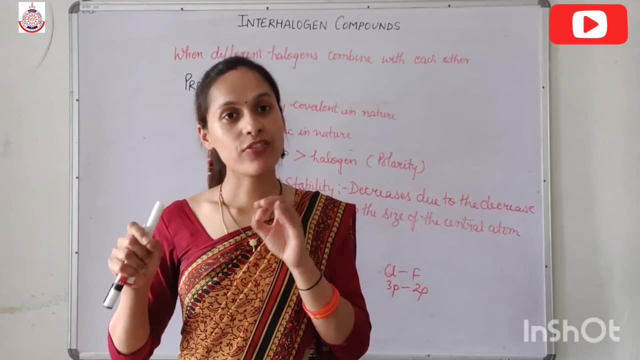 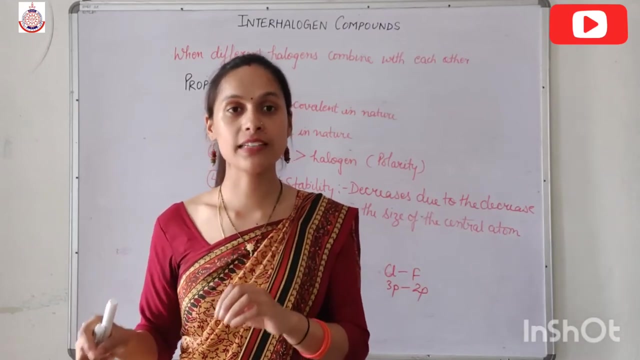 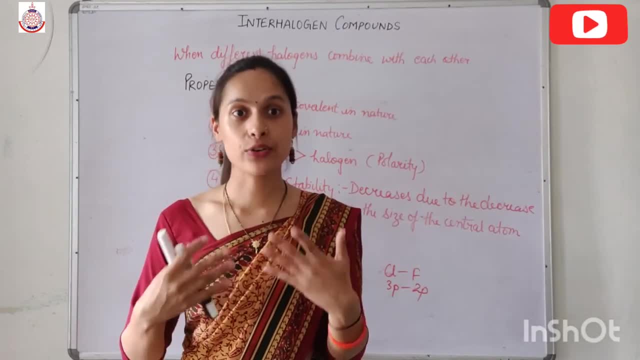 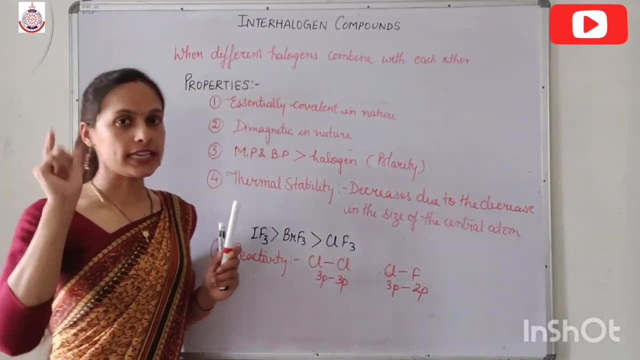 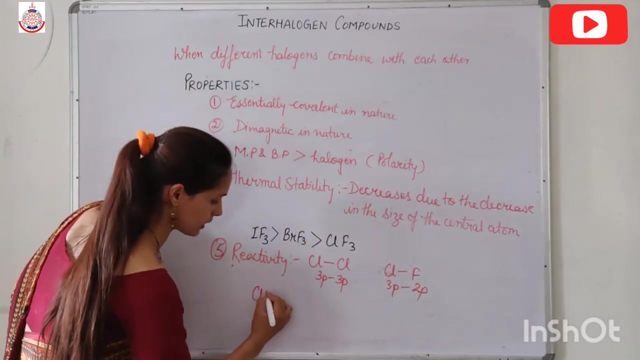 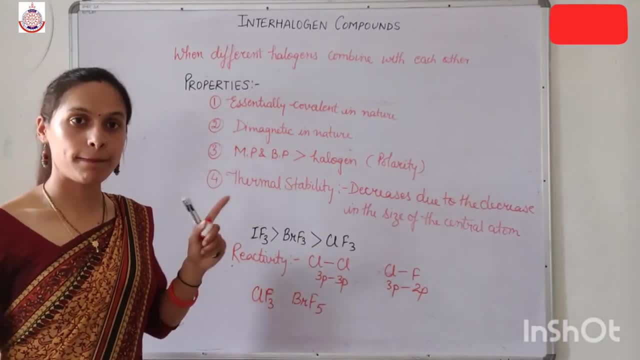 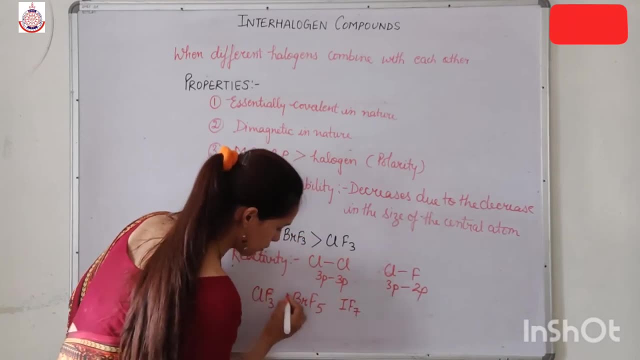 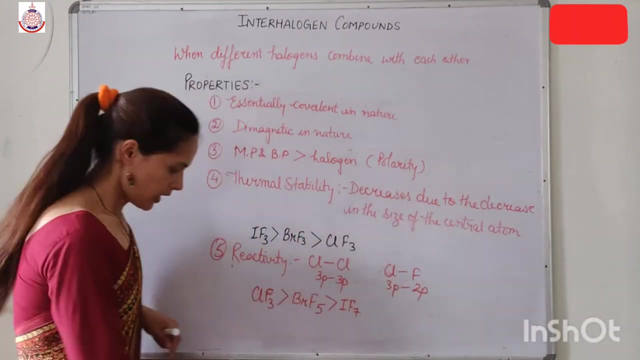 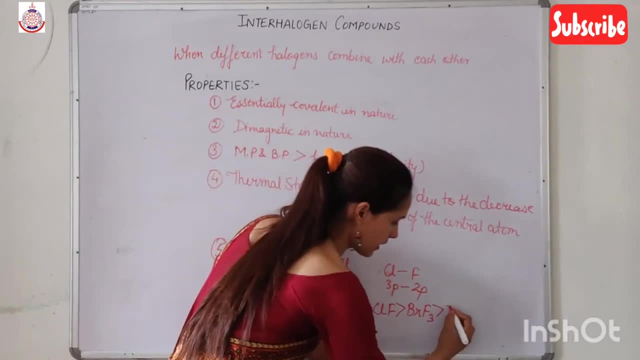 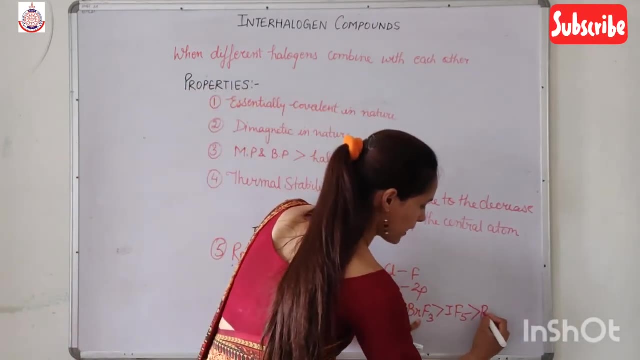 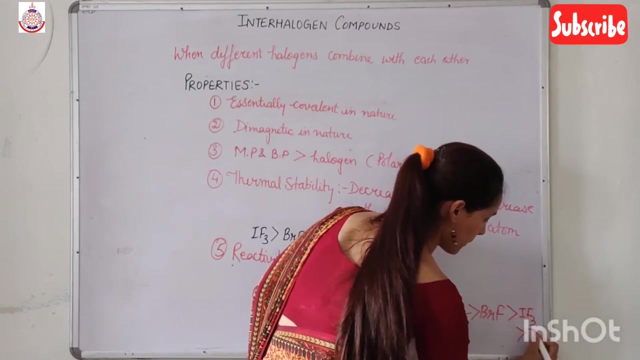 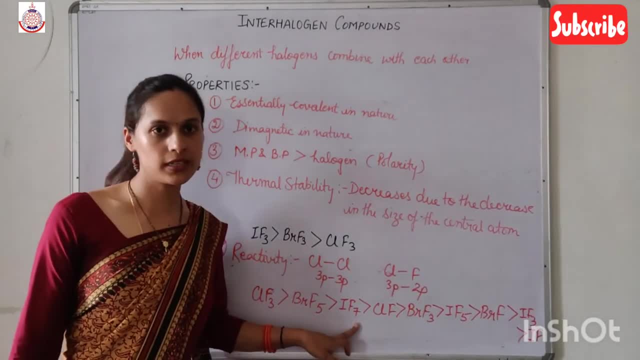 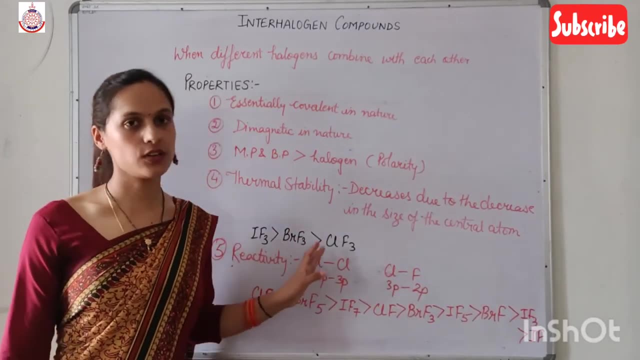 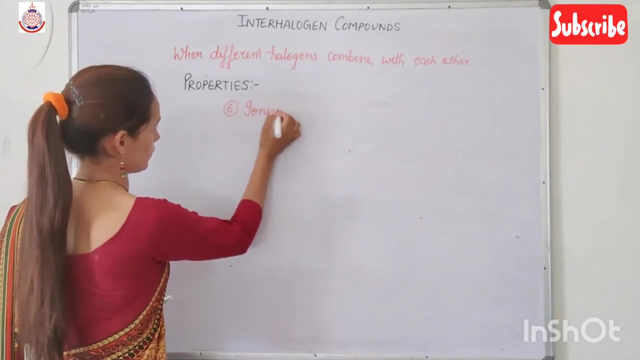 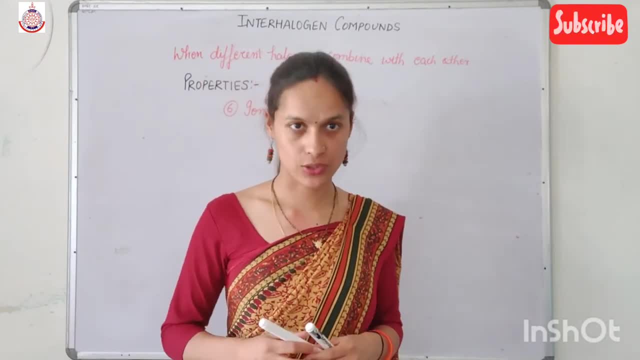 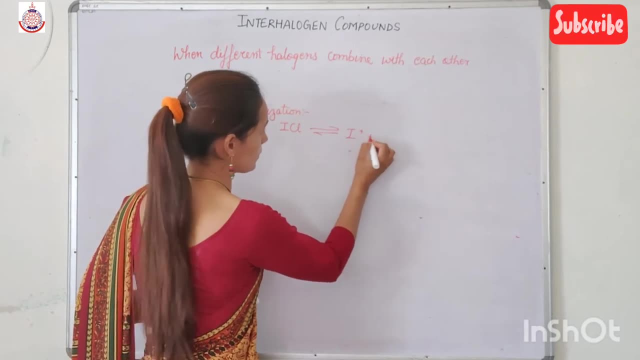 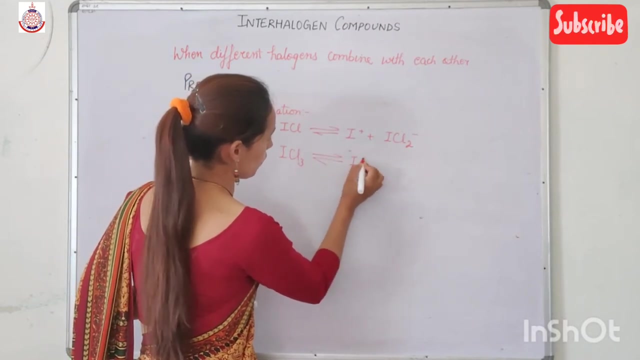 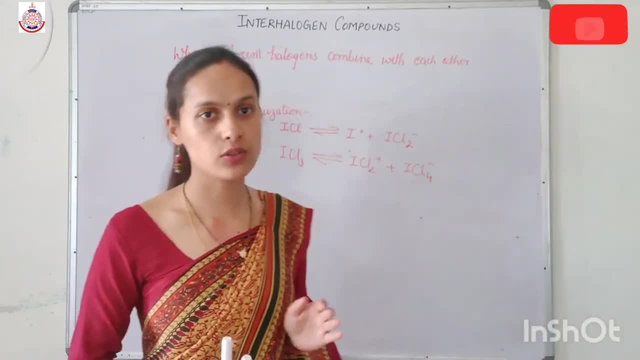 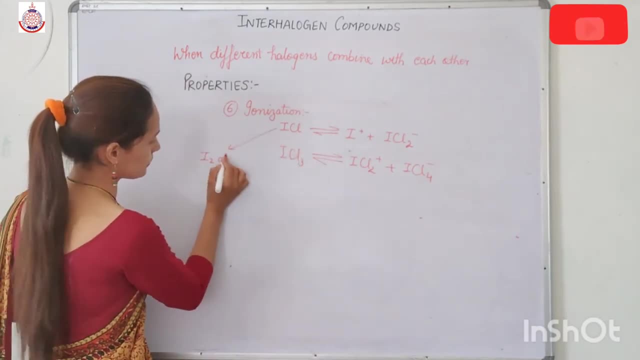 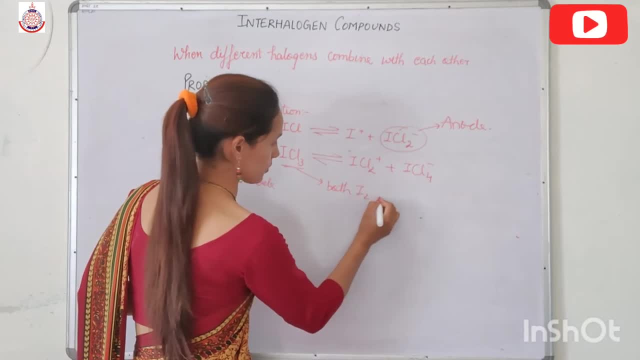 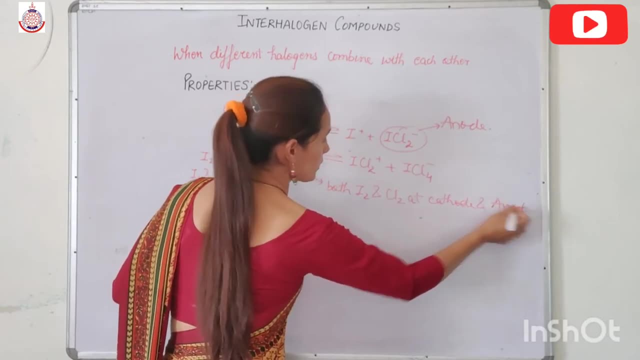 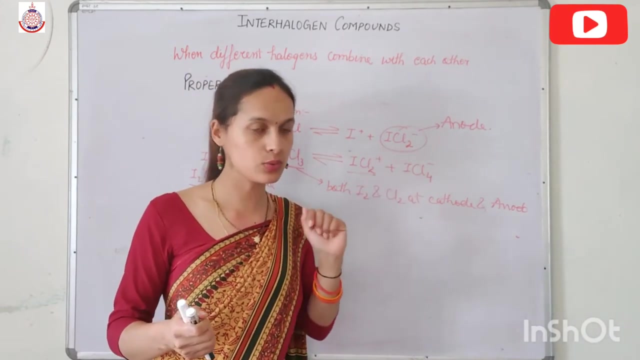 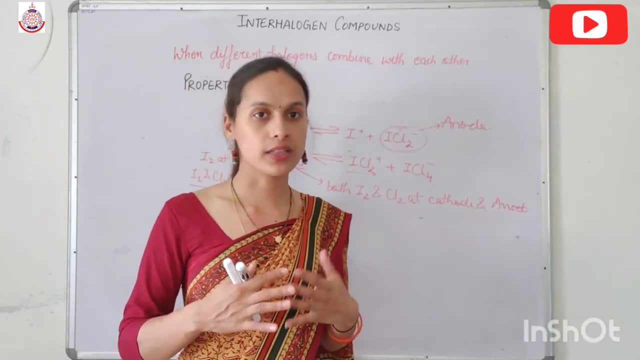 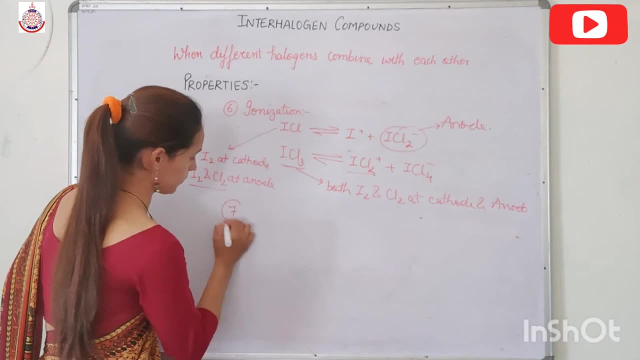 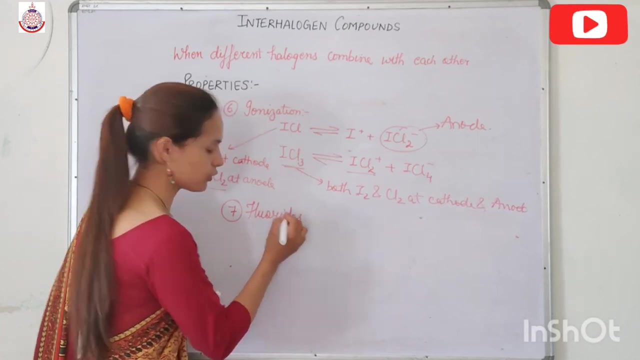 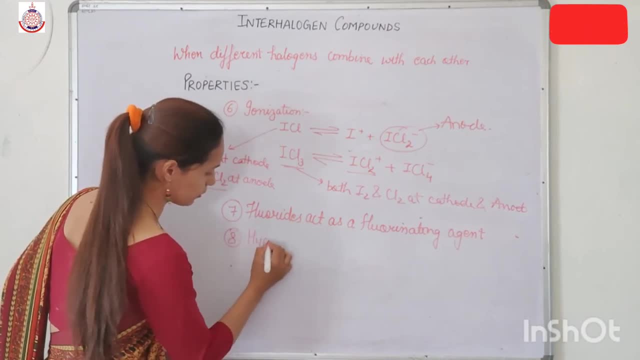 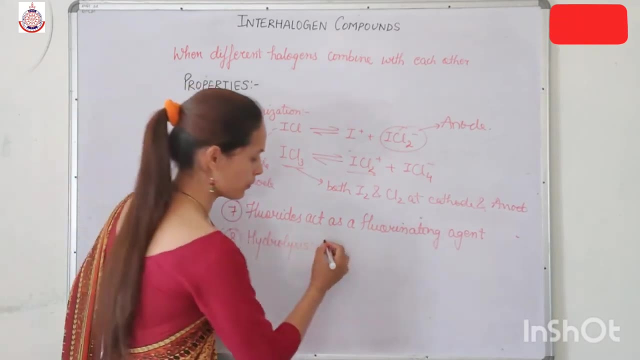 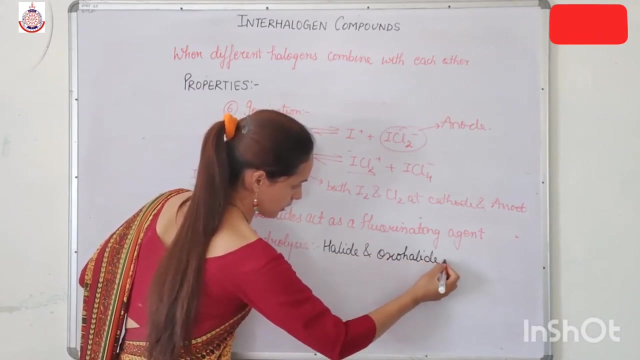 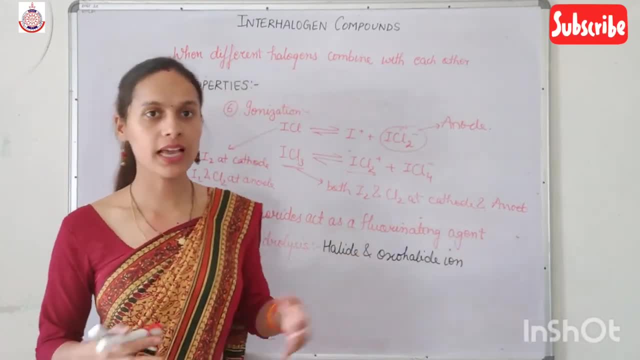 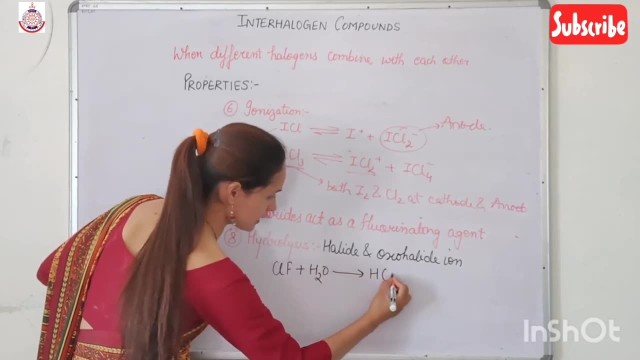 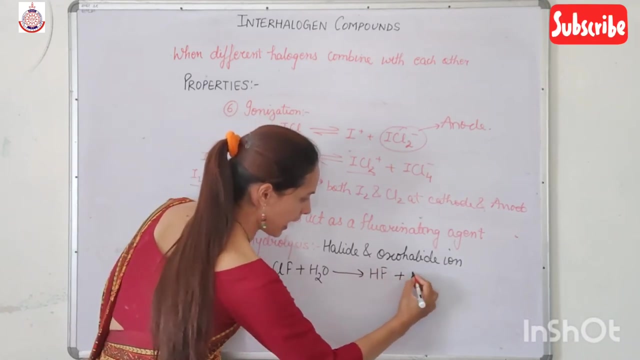 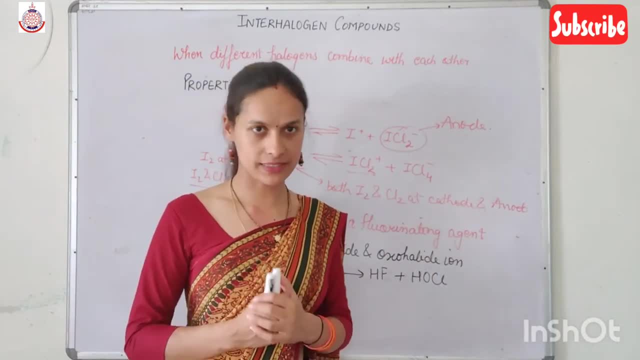 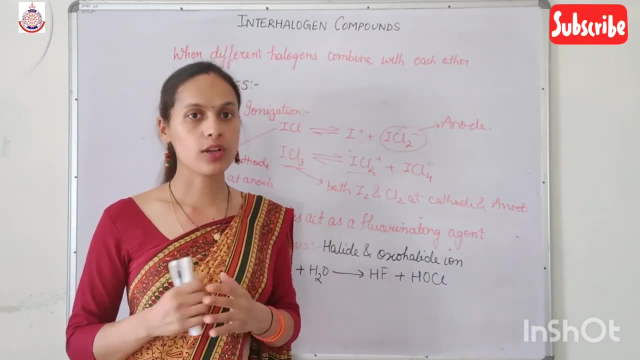 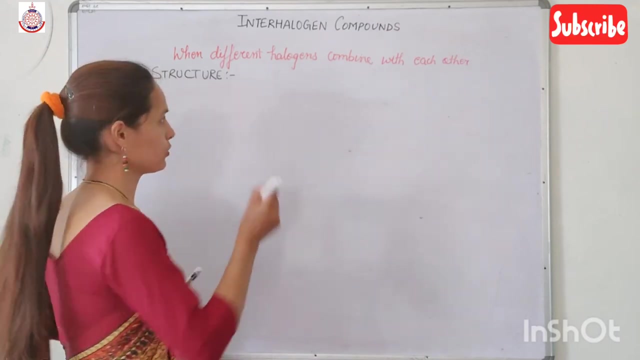 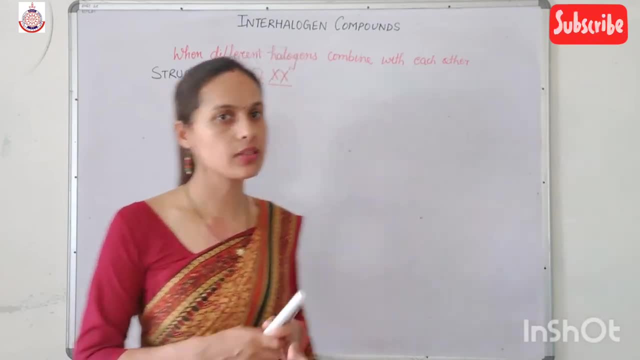 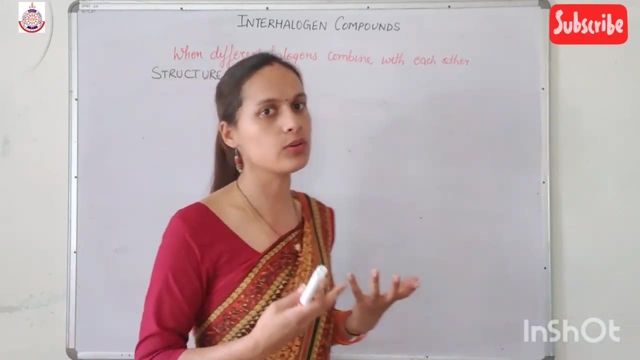 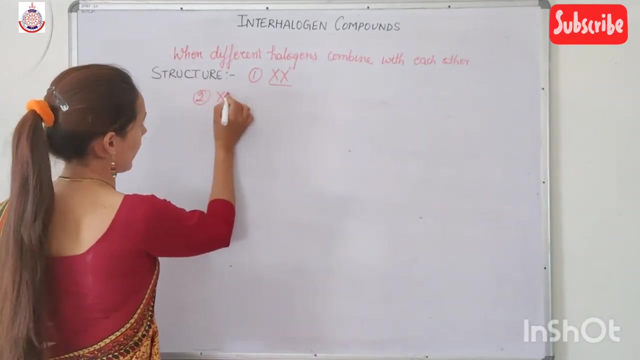 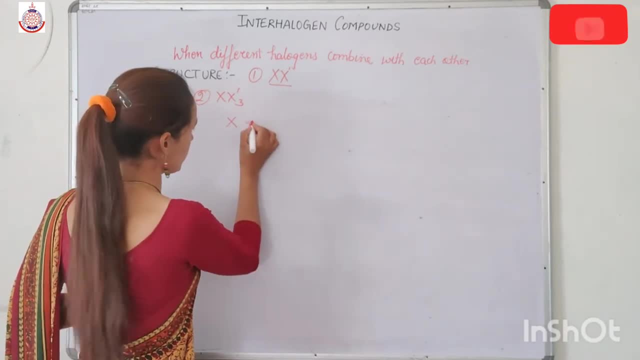 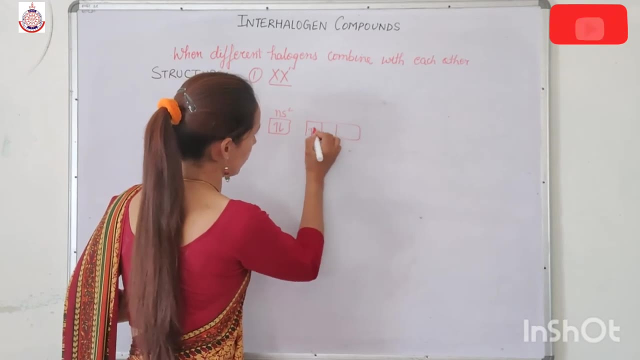 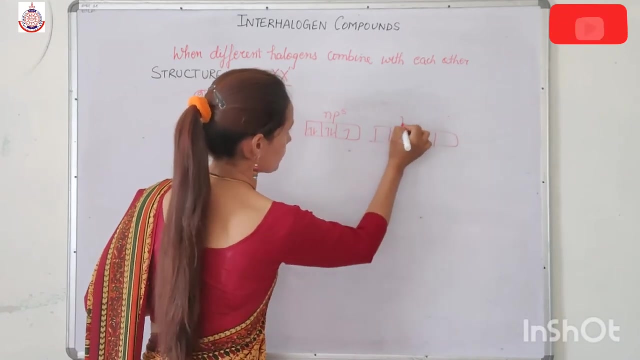 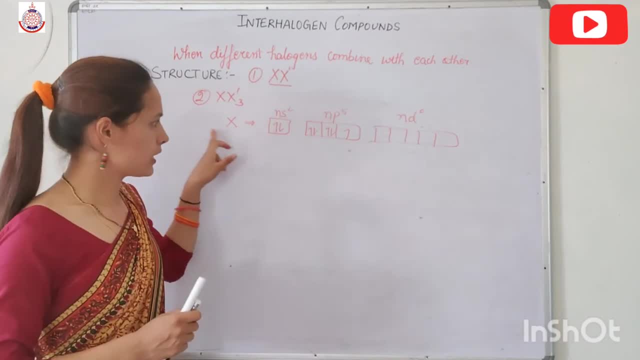 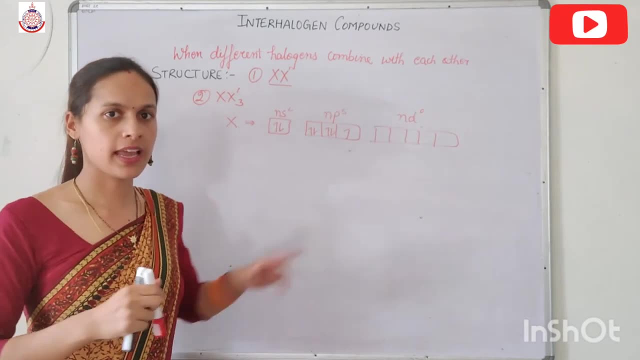 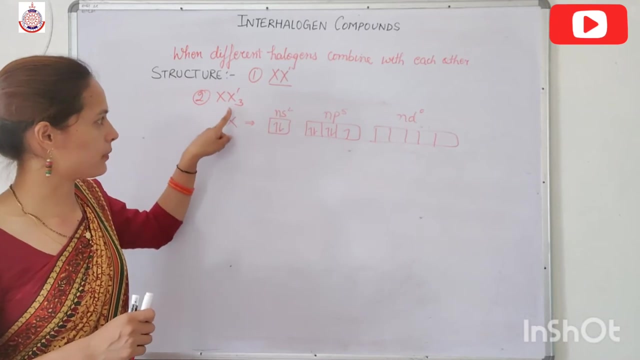 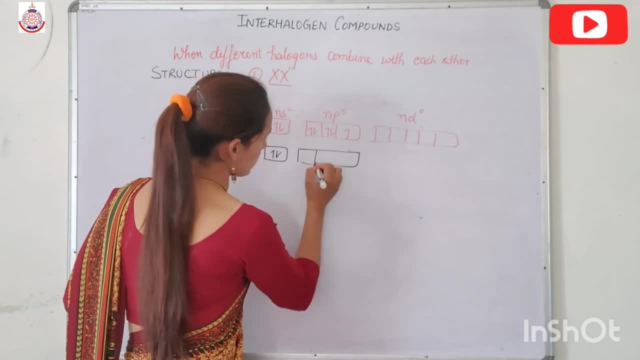 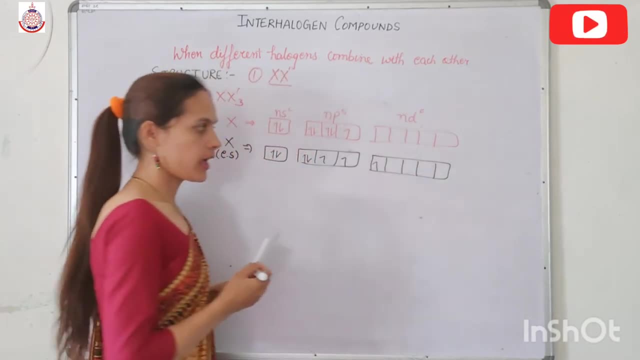 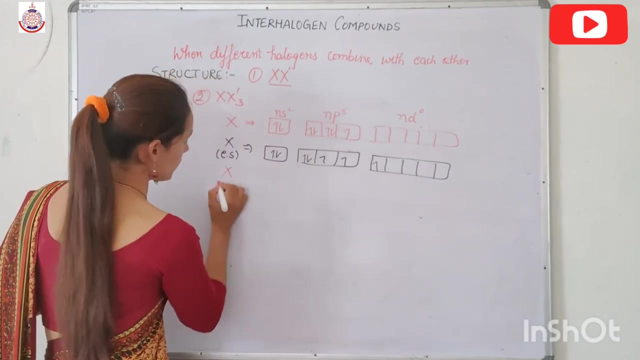 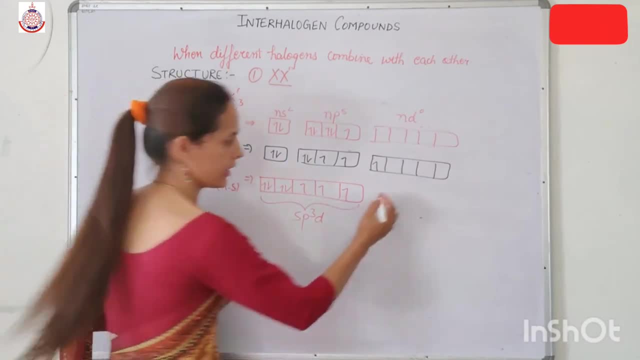 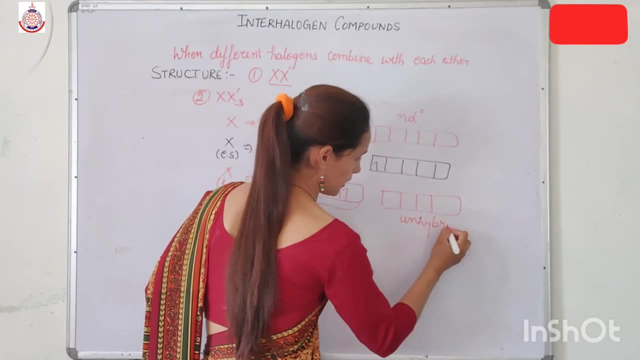 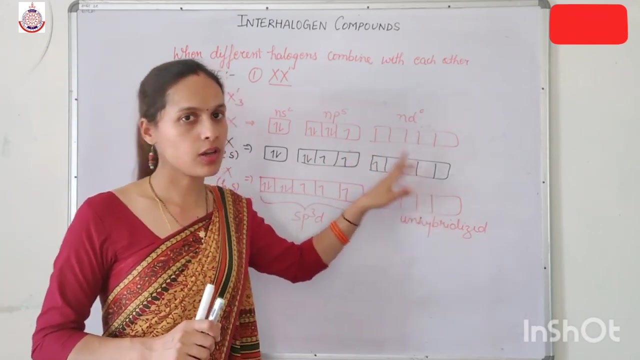 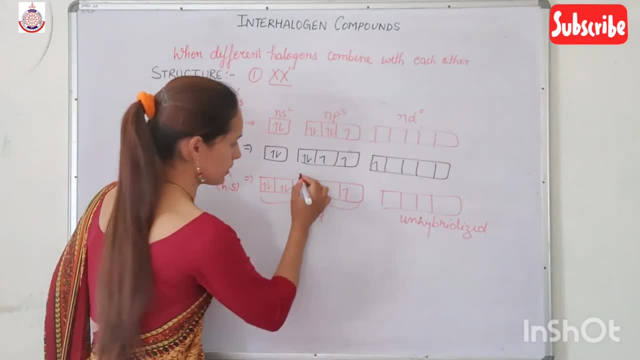 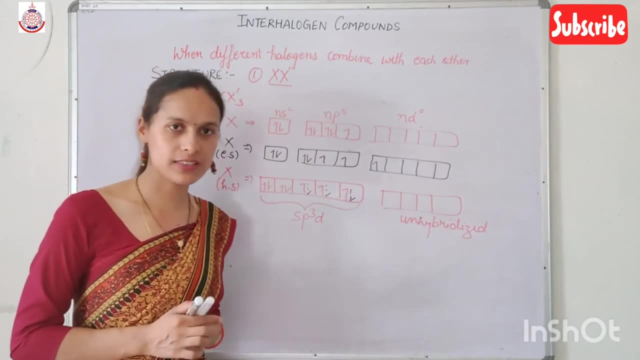 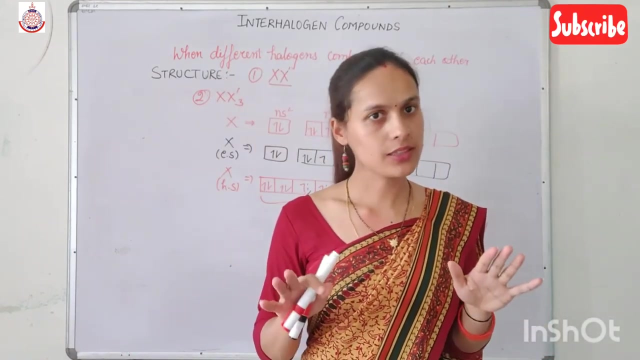 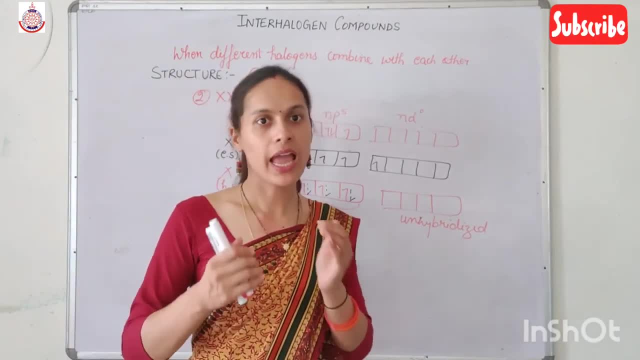 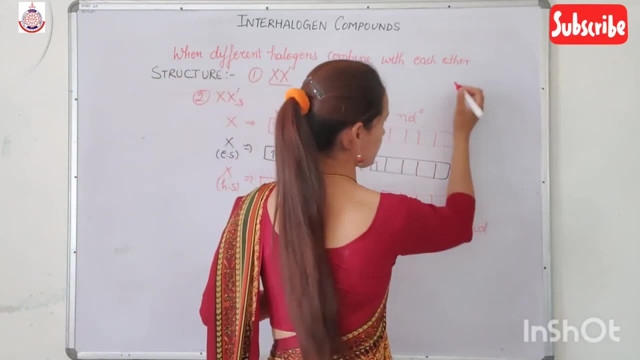 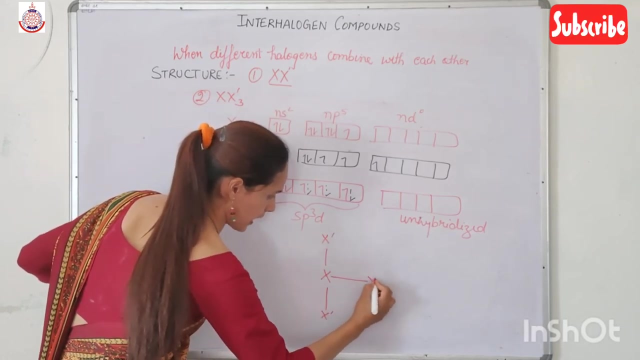 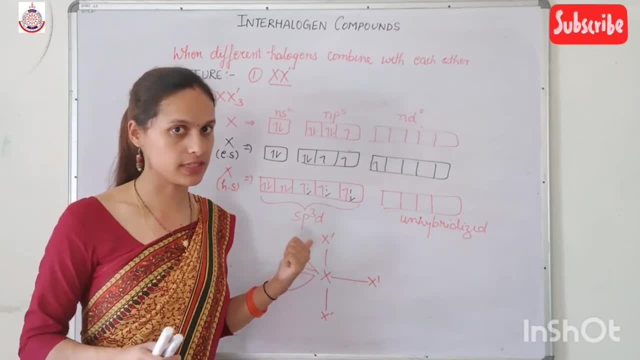 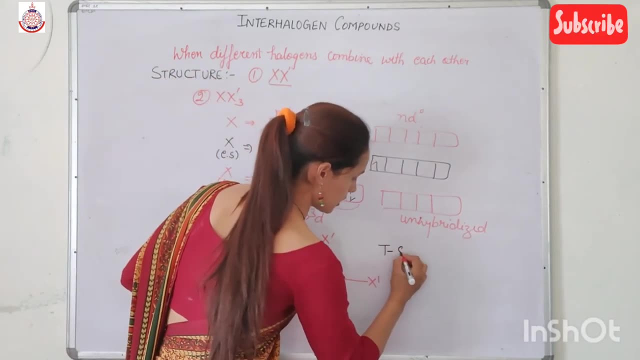 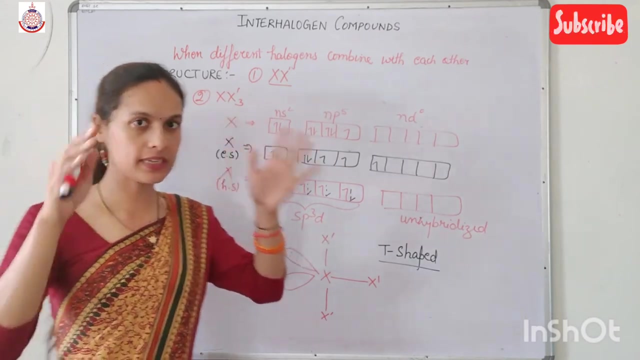 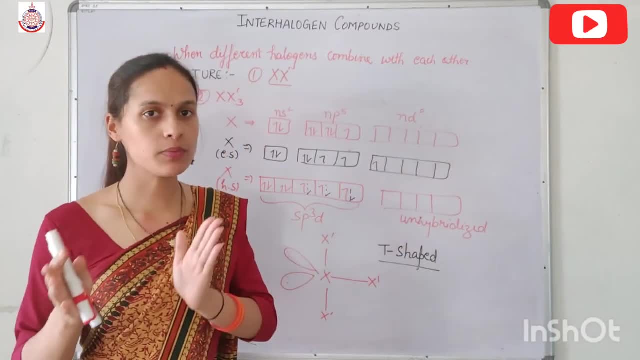 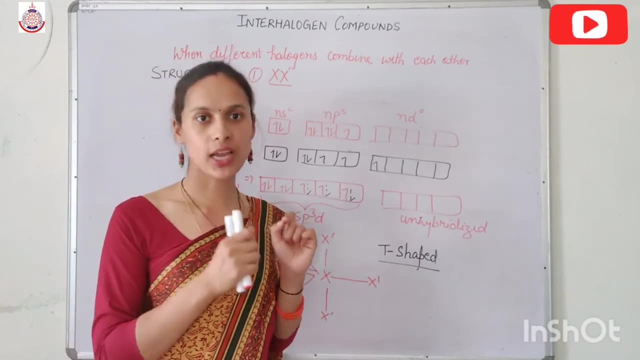 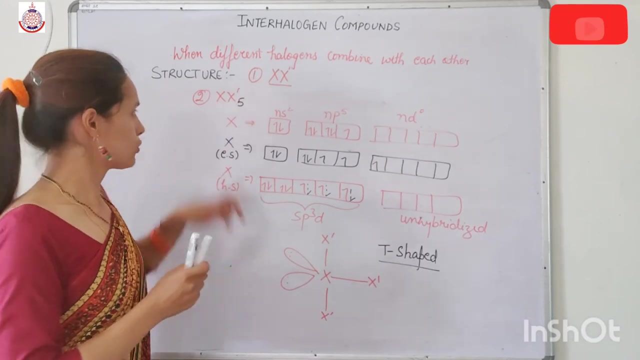 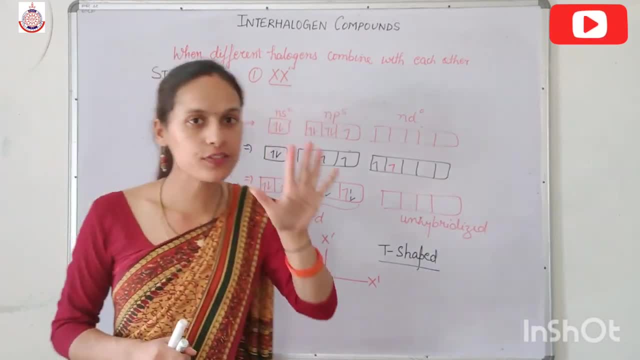 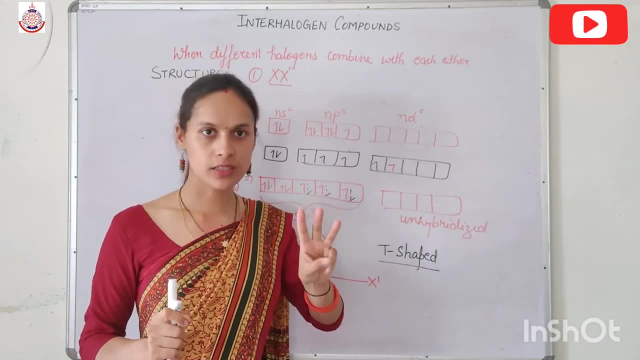 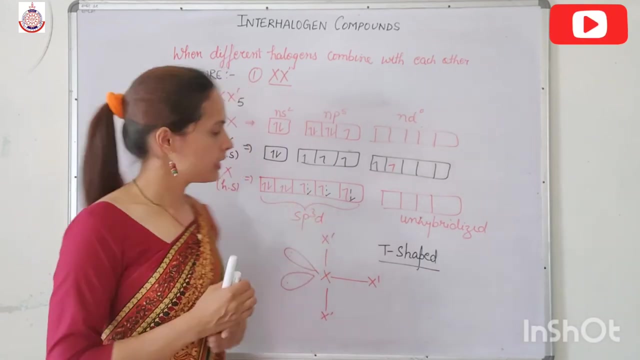 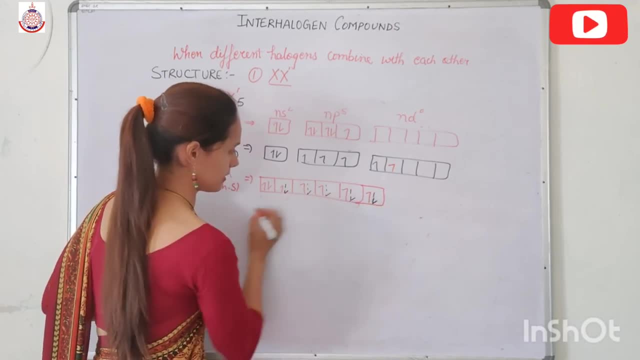 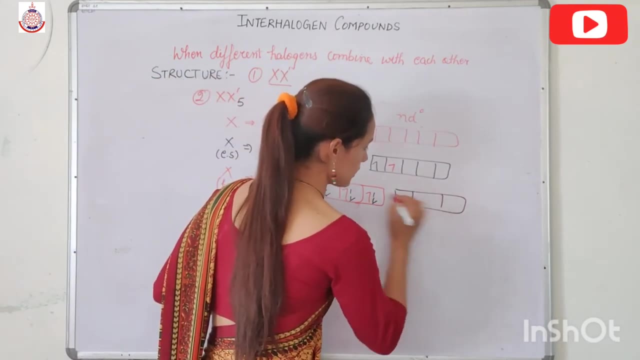 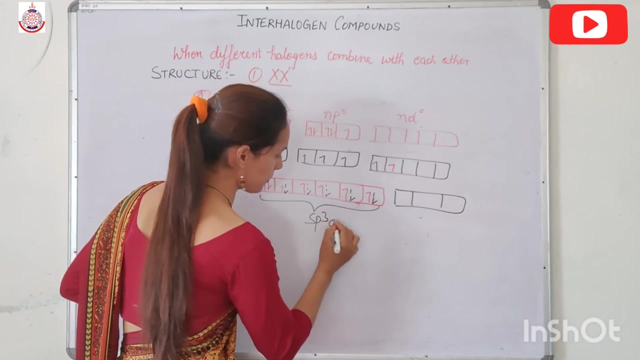 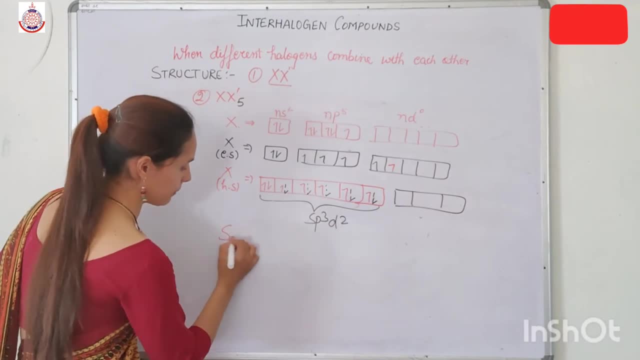 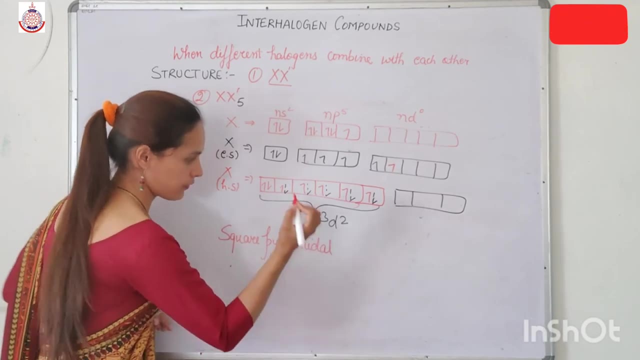 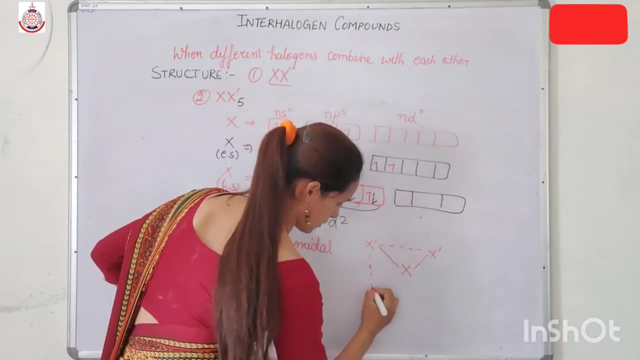 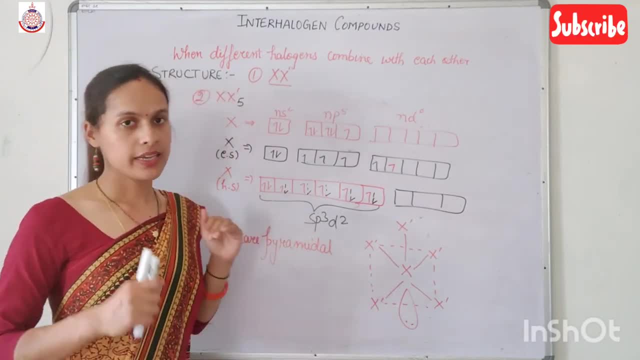 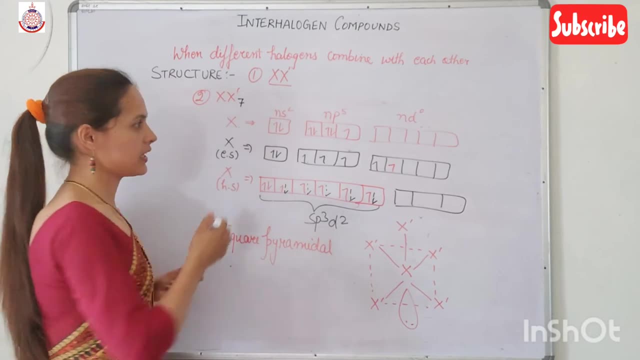 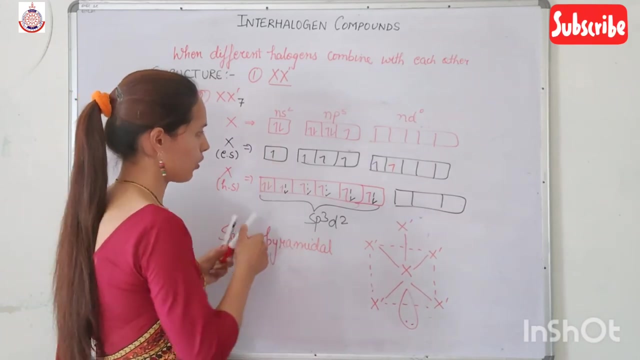 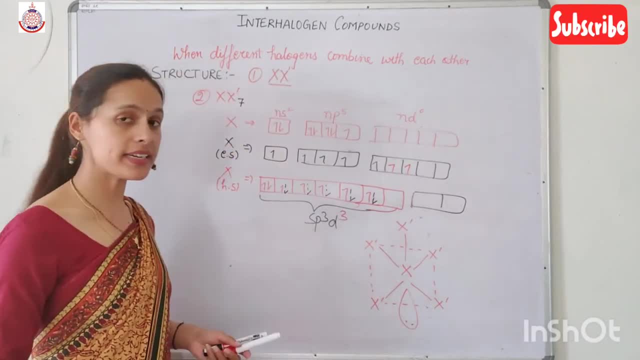 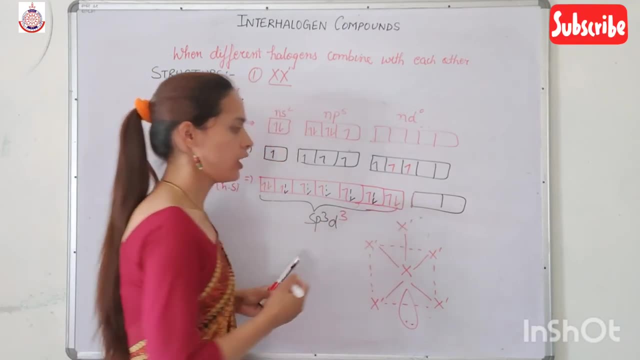 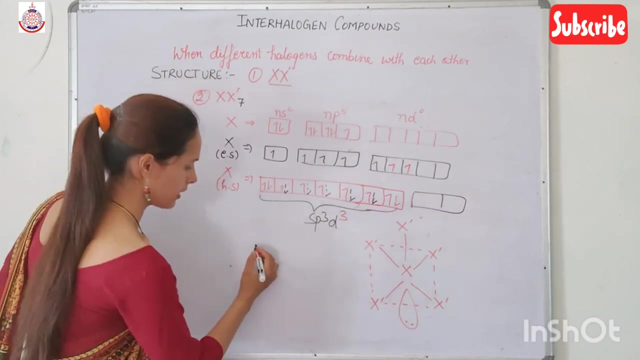 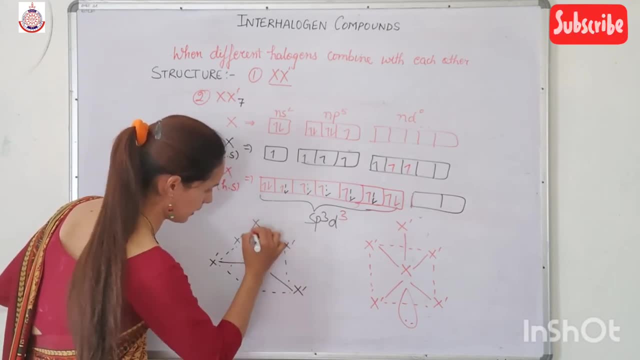 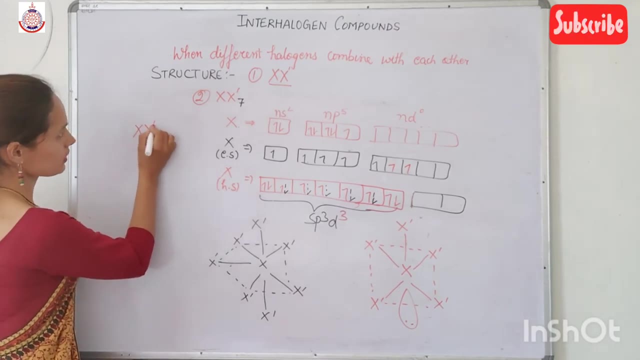 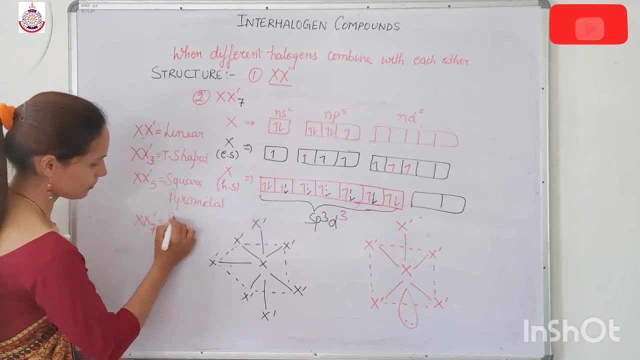 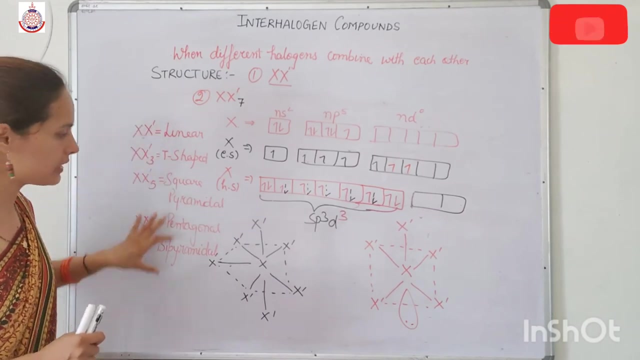 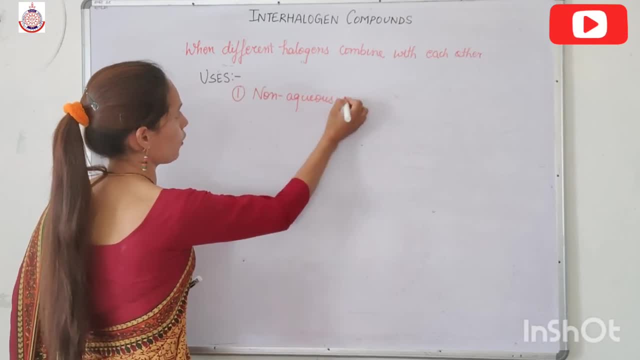 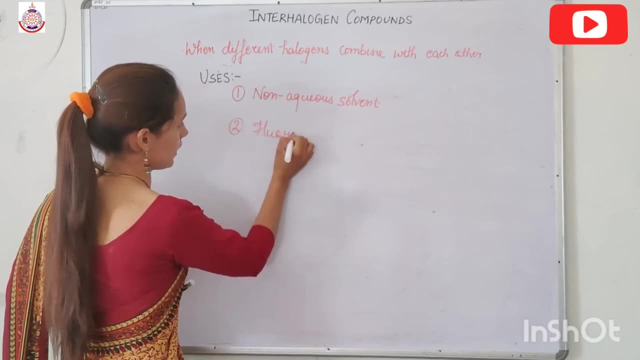 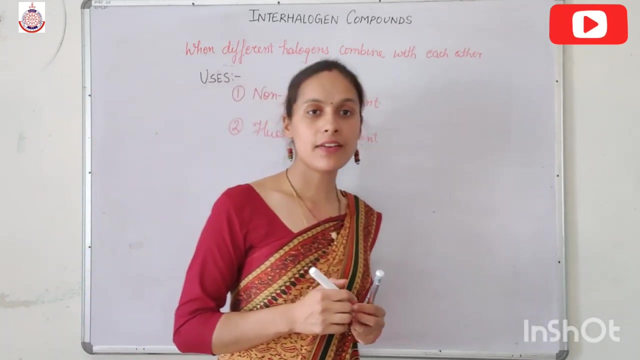 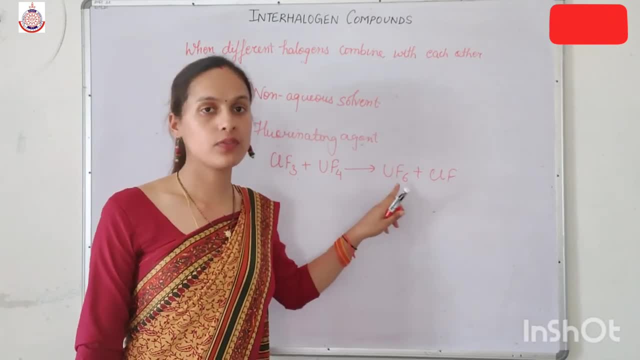 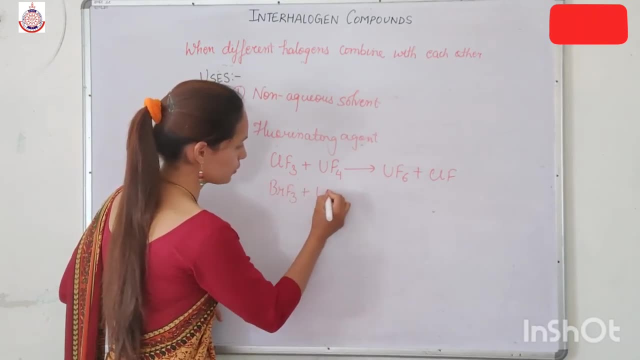 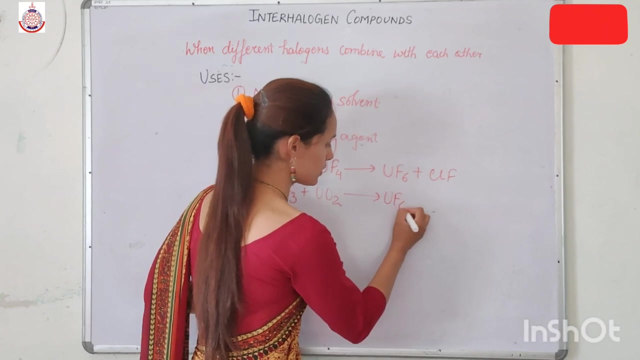 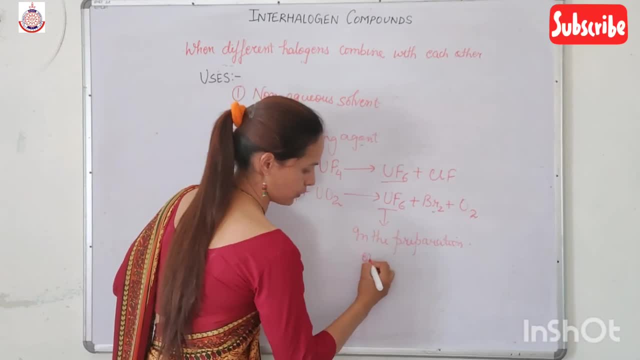 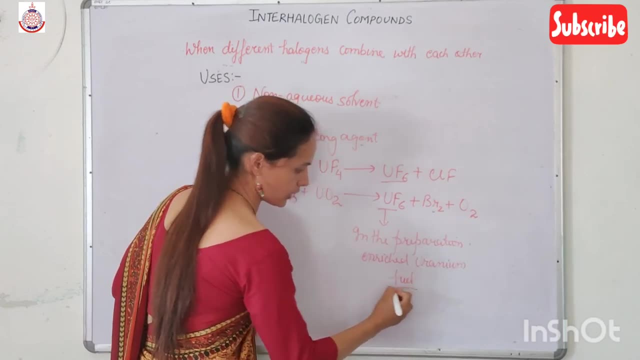 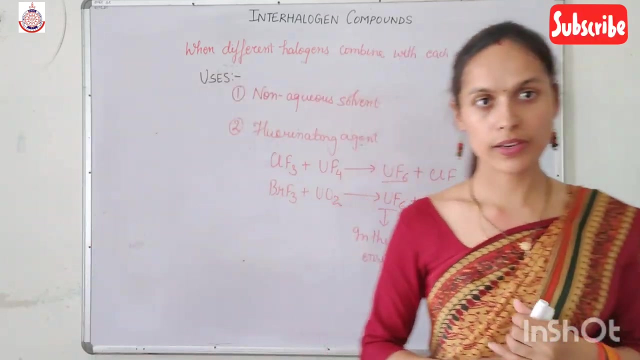